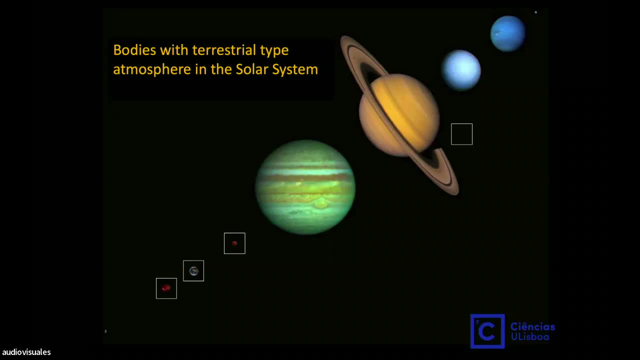 the bodies with the square are the only bodies, The bodies with atmosphere, in the hydrostatic equilibrium in our solar system. Of course that now there is a bridge from our knowledge in the solar system and what we are still, we still have a lot to learn, of course, and to share this knowledge and this synergy with. 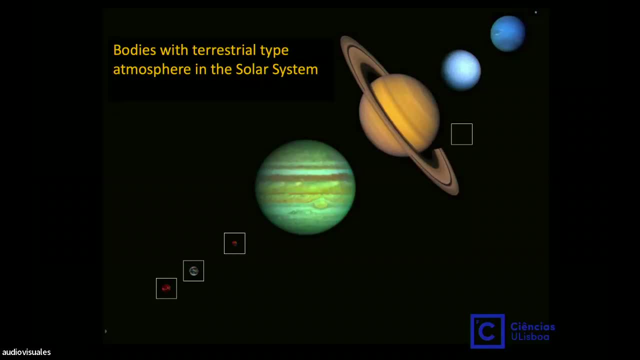 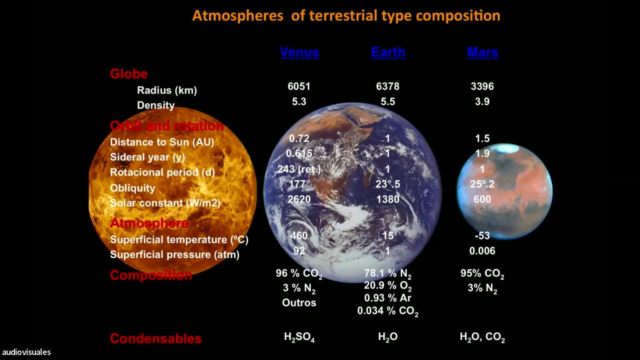 this new adventure that raised now, that began now, that is, the characterization of exoplanets atmospheres. So I will ask your attention for this table And I want to pinpoint here to you and I want to draw your attention for something here in this table. Just a couple of numbers, just one, some of them. 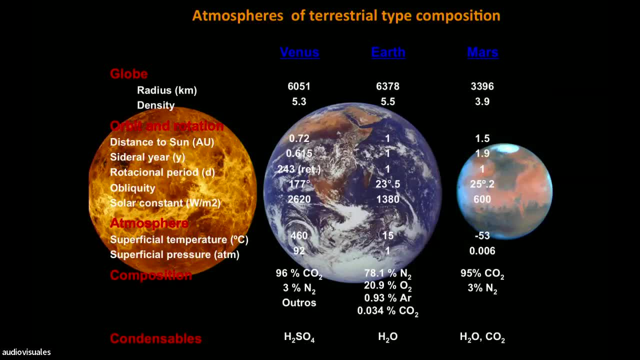 And but before I will give some context: if these planets, rocky planets, the telluric planets as Mars and Earth and Venus, therefore more or less at the same time and from, I would say, the same building blocks, from the planetary, never. 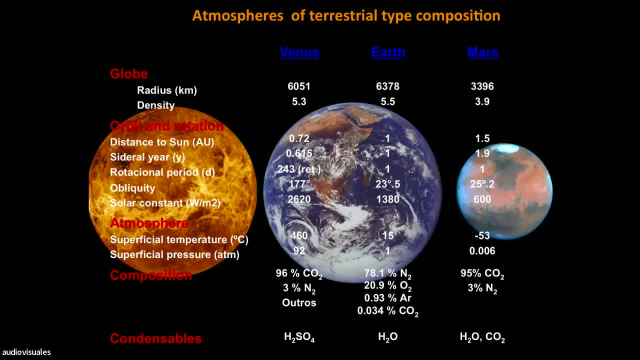 So I would say that the evolution of the primal planets must be quite similar And I would expect that The atmosphers in the beginning, the beginning They were quite similar- are and they evolve in such a different way. how come, why? let's see this, this history, and let's 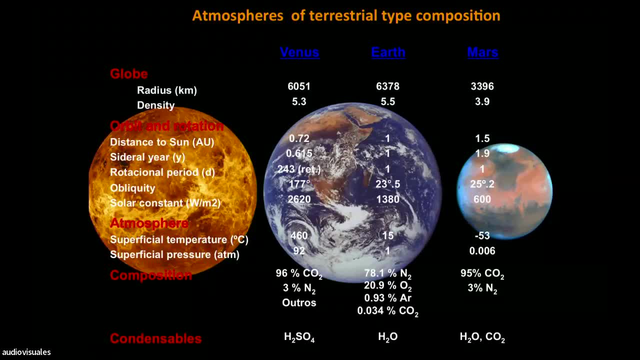 follow the water in this history, mostly- not just, but mostly- and usually we we used to say that, well, mars is so different from earth and venus is so different from earth. but i want to tackle this question in the other way around. is the earth that is quite different from the others? if not, 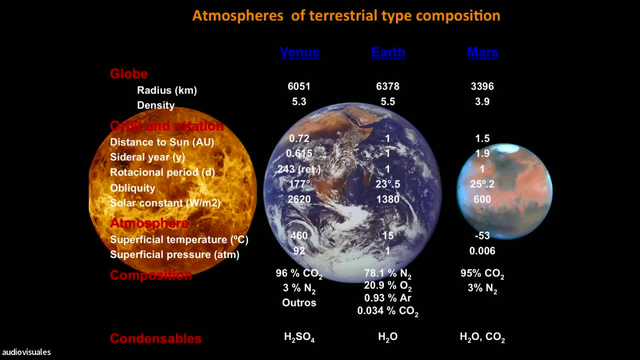 i want to draw your attention for the relative composition, and you can see here that the relative composition on mars, on vince, and on mars on co2 is almost the same and the, the, the, the nitrogen, on venus and mars is almost the same. so what is different in fact is earth, and as we and as we will see in the context a little bit, 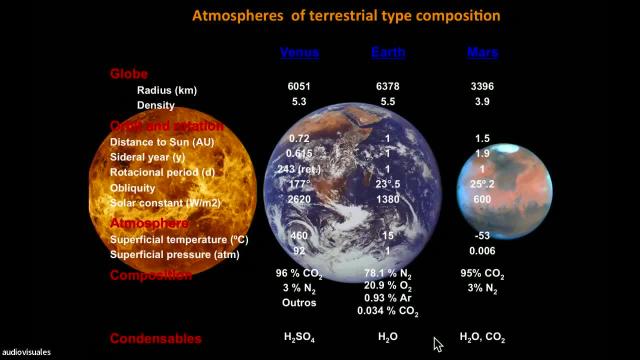 more specialized that we will see in the following slides. i would say that this is what. this is what i expected for the primordial atmospheres, that at least the relative composition was quite similar, as is still today- a rough approximation, of course, between venus and mars. 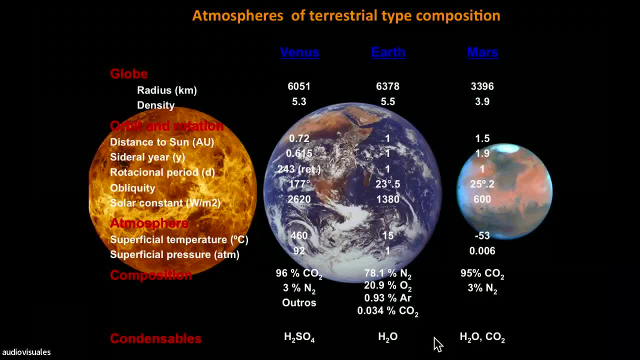 so what happened to us to evolve in such a different way? it's, of course, what we will see in the following. right now, most of you perhaps are thinking: yeah, but it's quite different to the, the atmosphere on mars and venus, of course, and they evolved in a in a such a different way and, as you know, the 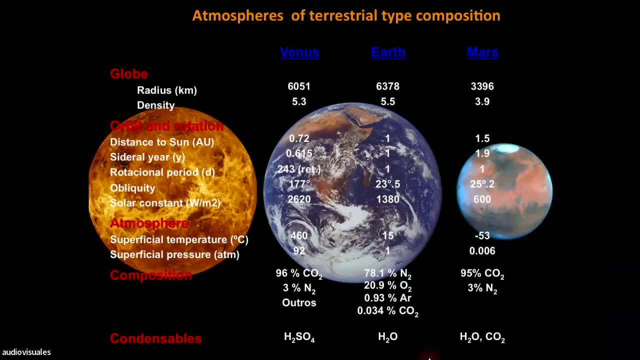 superficial pressure on venus today is like 22 bars, so it's like being one kilometer below the surface in the sea, so a soda can will smash with this pressure and the. the pressure at the surface on mars, as you well know, is less than one percent of our own earth. so what? how come? why did it evolve? 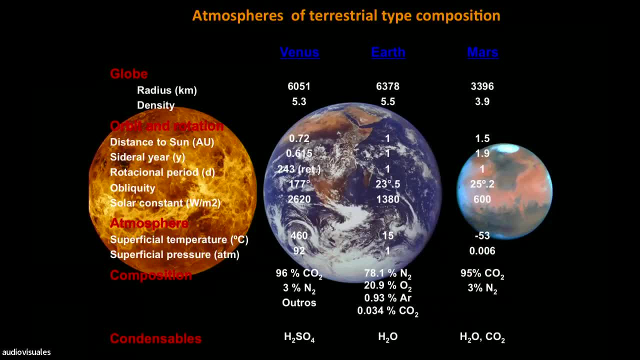 in such a different way, and also the superficial temperature is another thing that i want and we will discuss today- is more than 460 degrees plumb will melt at this surface temperature on venus and on mars- very low. well, so let's see what provoked this, this uh other different uh cases in the temporal evolution between venus and. 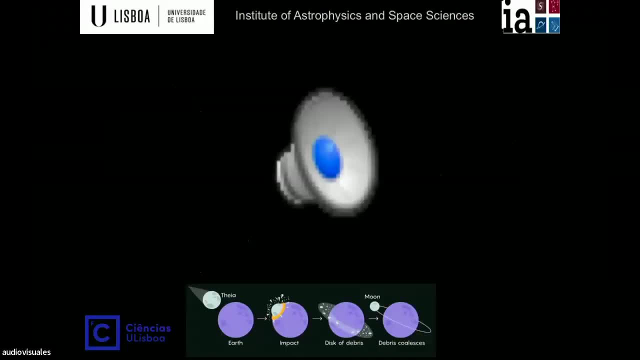 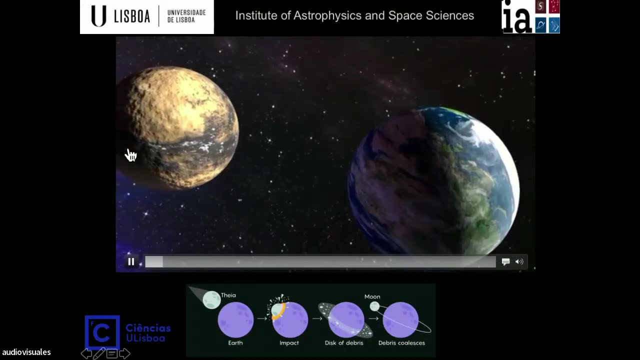 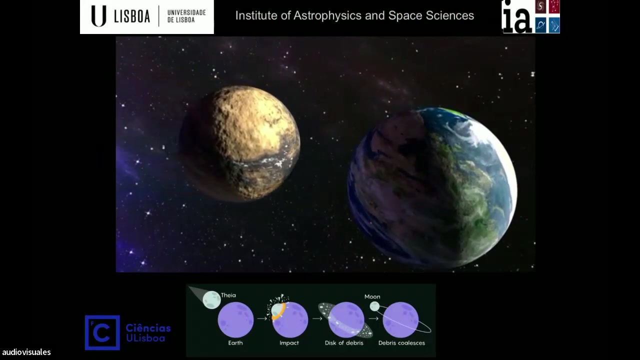 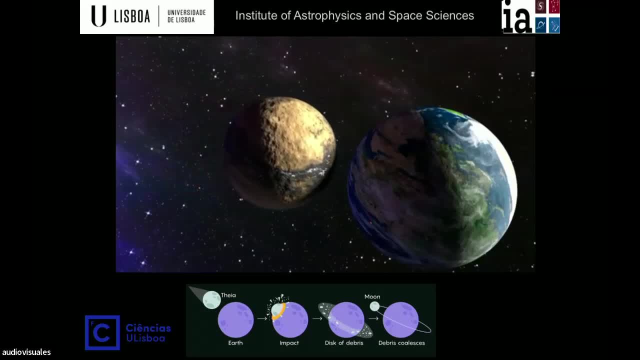 that comes in the books for a long time, for a long time, for a long time. and you are specialized on this topic. so you and you are specialized on this topic, so you and you are specialized on this topic. so you know, know, know, most of you better than me. 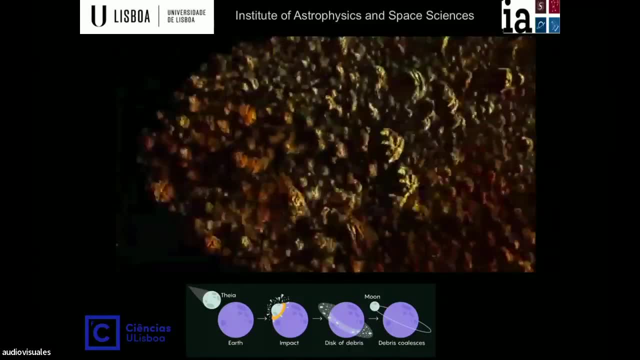 most of you better than me, most of you better than me. that that that well, well, well, this with this collision with today, this with this collision with today, this with this collision with today, it's something that we all know. it's something that we all know. it's something that we all know. the new thing: 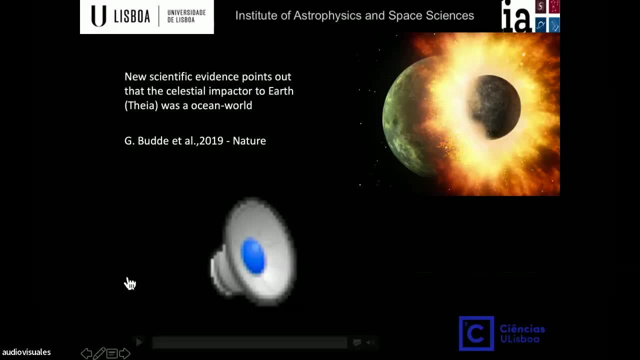 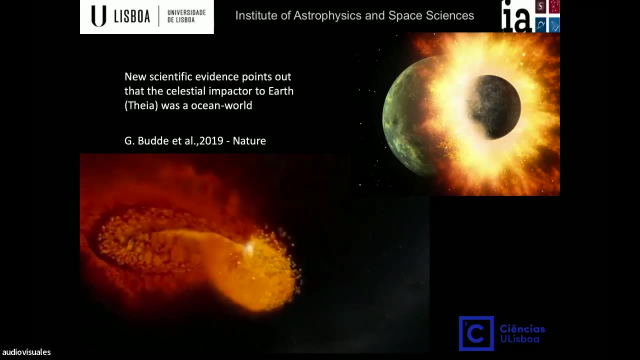 the new thing, the new thing is the most, the new thing is the most, the new thing is the most: new evidence about new evidence, about new evidence about uh from buddha at all from 2019 nature. uh from buddha at all from 2019 nature. 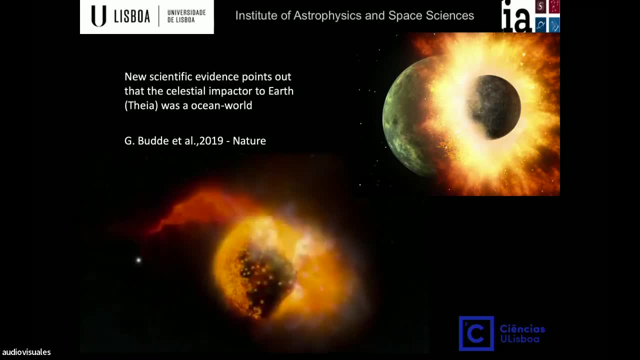 uh, from buddha at all, from 2019, nature. is that his impactor was in fact? is that his impactor was in fact? is that his impactor was in fact not an irregular asteroid, not an irregular asteroid, not an irregular asteroid, but the ocean worlds. 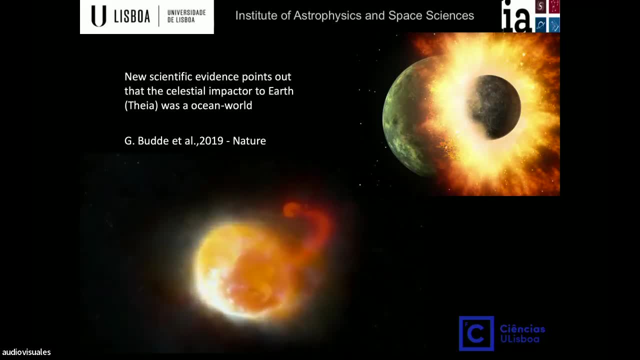 but the ocean worlds, but the ocean worlds. based on isotopic ratios in the. based on isotopic ratios in the. based on isotopic ratios in the overage of isotopes like molybdenum. overage of isotopes like molybdenum. 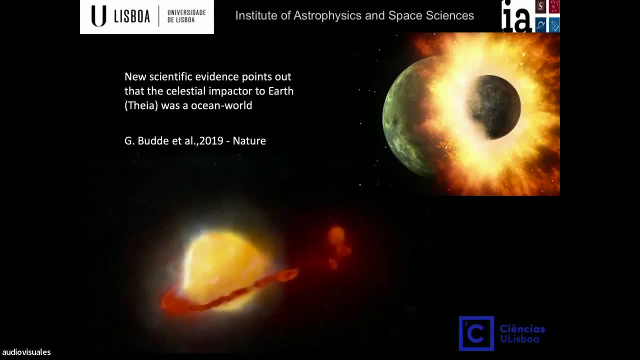 overage of isotopes like molybdenum, and so the thing is that we have an. and so the thing is that we have an, and so the thing is that we have an abort of an extra amount of water, that abort of an extra amount of water that 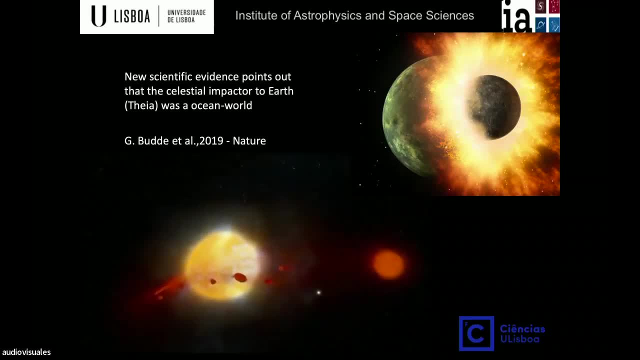 abort of an extra amount of water that was immense, was immense, was immense on earth and on earth and on earth. and of course that will tackle a lot of, of course that will tackle a lot of, of course that will tackle a lot of different systems, as we will see on the 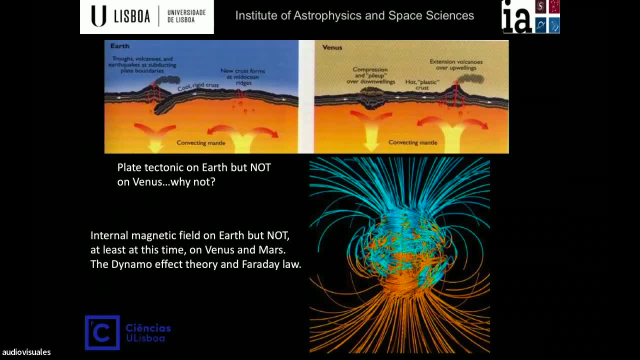 different systems, as we will see on the different systems, as we will see on the phone first, phone first, phone first, we will have an extra water and we will have an extra water and we will have an extra water and uh, water like oceans are like sponge. uh, water like oceans are like sponge. 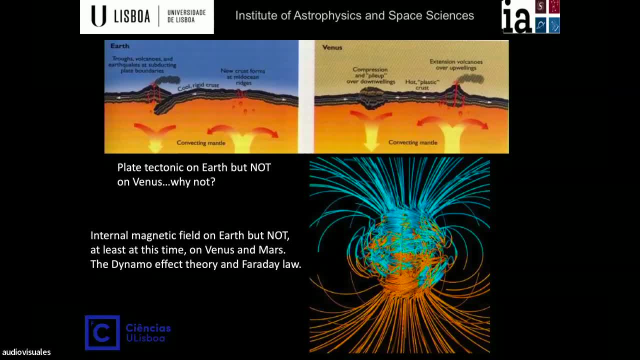 uh, water, like oceans, are like sponge for co2. that we all know for co2. that we all know for co2, that we all know that now, that now that now we expect that we expect that we expect that that starts the main difference in the, that starts the main difference in the. 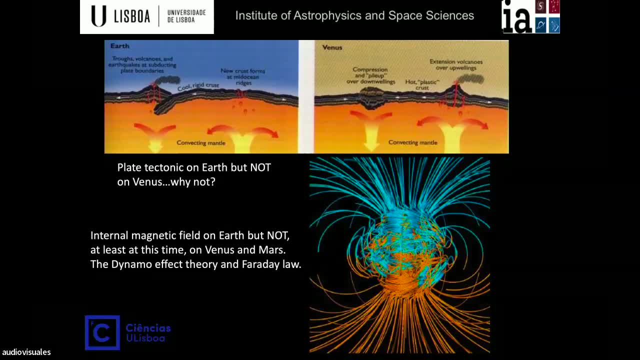 that starts the main difference in the temporal evolution of first temporal evolution of first temporal evolution of first, that was most of that co2. that was. that was most of that co2. that was. that was most of that co2 that was grabbed by oceans, grabbed by oceans. 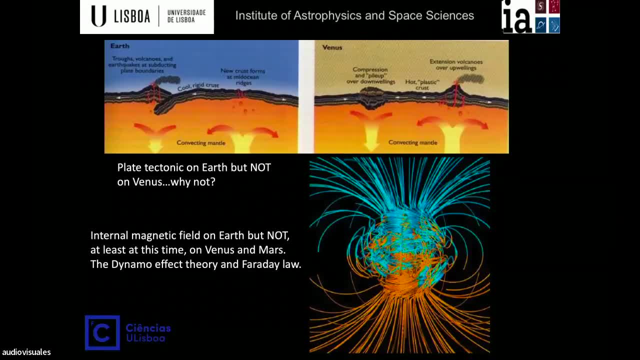 grabbed by oceans in the first step, but there are other in the first step, but there are other in the first step, but there are other steps, steps, steps, and the other step is that we'll have, and the other step is that we'll have, and the other step is that we'll have an extra amount of water in the crust. 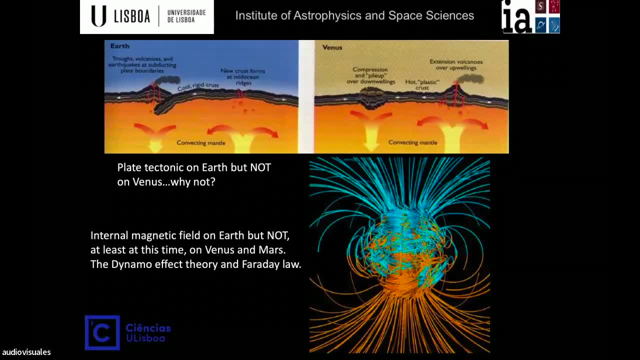 an extra amount of water in the crust, an extra amount of water in the crust, so, and this water will work as a so, and this water will work as a so, and this water will work as a lubricant, lubricant, lubricant, so it will be much easier to. 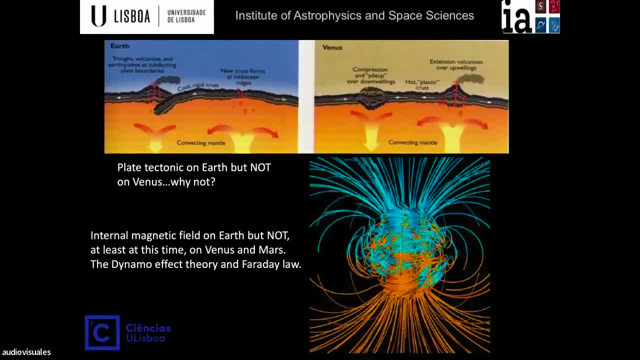 so it will be much easier to. so it will be much easier to layers, layers, layers to to, to move, move, move between them, so between them, so between them. so will be much easier. so less friction will be much easier. so less friction will be much easier, so less friction to have. 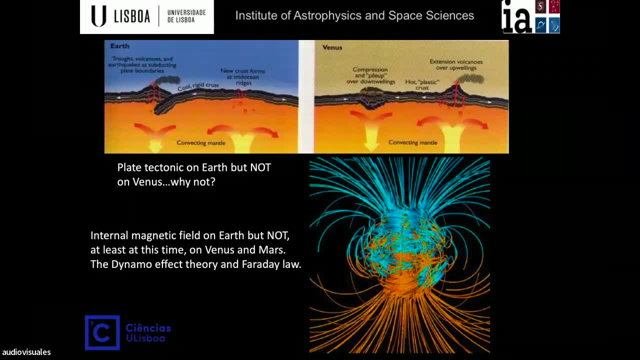 to have to have: click, oh sorry here, click, oh, sorry here, click, oh sorry here. that's yeah, yeah, yeah, so, so, so we'll have, we'll have, we'll have uh less, uh, less, uh, less, less friction, and so we will have less less friction, and so we will have. 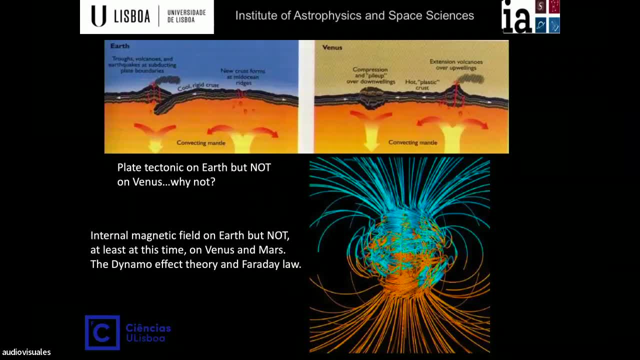 less, less friction, and so we will have that, that, that uh plate tectonics that will uh, uh uh remove this extra co2. that was remove this extra co2, that was remove this extra co2 that was delivered for to the crust, delivered for to the crust. 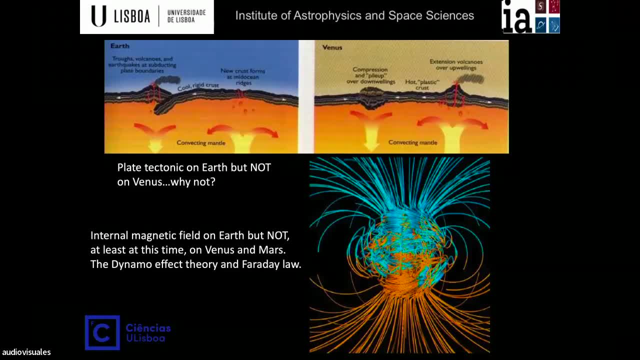 delivered for to the crust, to beneath the subsurface subsurface, to beneath the subsurface subsurface, to beneath the subsurface subsurface, bearing this extra co2, bearing this extra co2, bearing this extra co2. if we go back to that, if we go back to that, 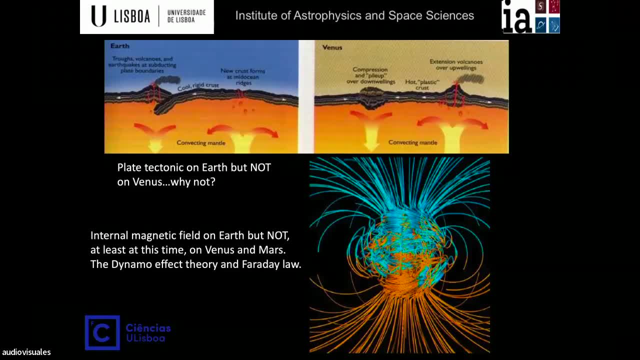 if we go back to that slide where i had this table with slide where i had this table with slide, where i had this table with different numbers, different numbers, different numbers, the extra amount of atmospheric mass, the extra amount of atmospheric mass. the extra amount of atmospheric mass was, if you remember, mostly co2, but 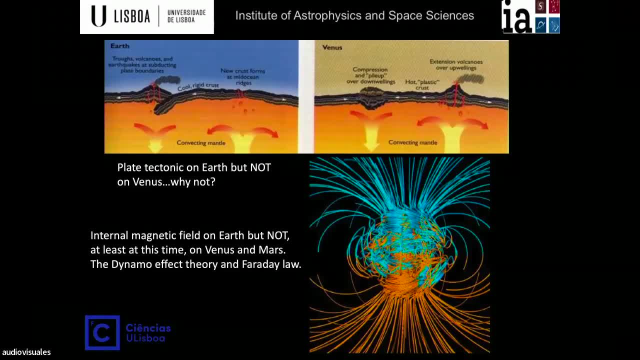 was, if you remember, mostly co2, but was, if you remember, mostly co2. but if we bury the co2, if we bury the co2, if we bury the co2 in the beneath the surface, we will in the beneath the surface, we will in the beneath the surface, we will will remove from the atmosphere a great 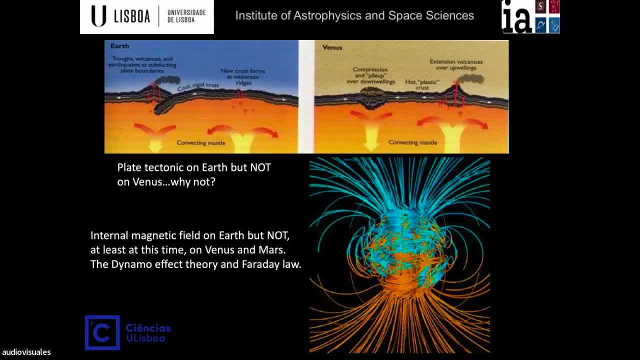 will remove from the atmosphere a great will remove from the atmosphere a great deal of mass, deal of mass, deal of mass. so now is easier to understand why in so now is easier to understand why in so now is easier to understand why in the temporal evolution, the temporal evolution, 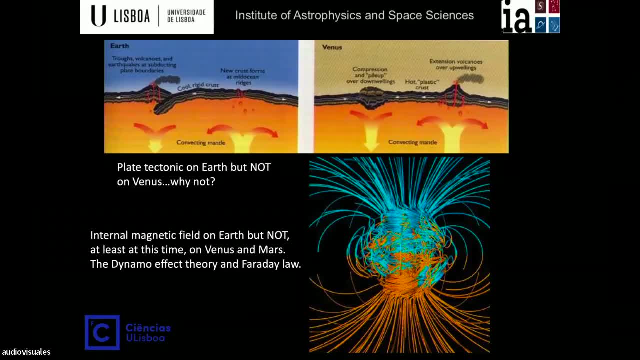 the temporal evolution between venus and earth, the between venus and earth, the between venus and earth, the. the quantity of atmospheric gazes. the quantity of atmospheric gazes. the quantity of atmospheric gazes on venus is much on venus is much on venus is much higher than on earth. but because 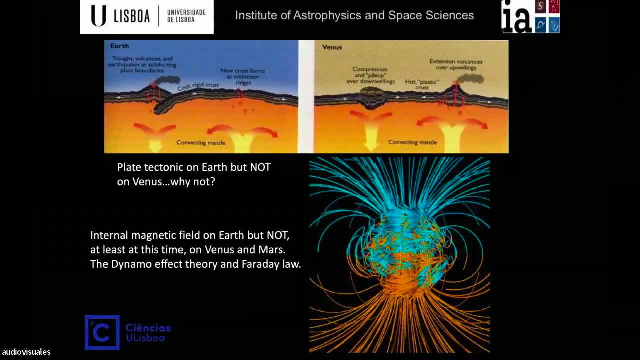 higher than on earth, but because higher than on earth, but because the initial conditions were similar. the initial conditions were similar. the initial conditions were similar: the mass of the mass of the mass of earth and winds quite similar as you. earth and winds quite similar as you. earth and winds quite similar. as you know, we often call 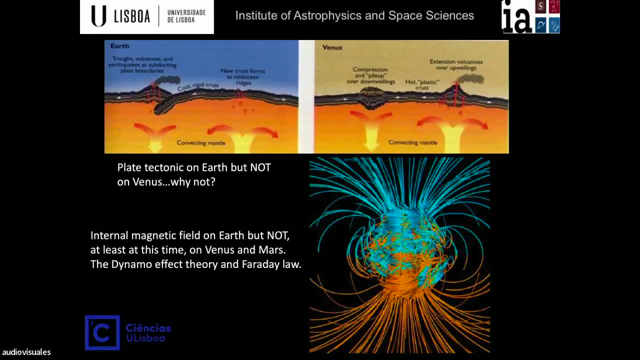 know we often call, know we often call to venus, the evil twin of earth, to venus, the evil twin of earth, to venus, the evil twin of earth. and now we understand one of the things, and now we understand one of the things, and now we understand one of the things that 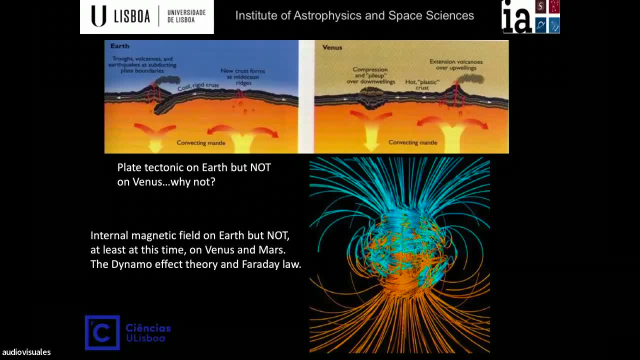 that that made the, made the made the, this global difference in the temporal, this global difference in the temporal, this global difference in the temporal. evolution. so evolution, so evolution. so we have the emotion, we have the emotion, we have the emotion that we removed a lot of, a great deal of. 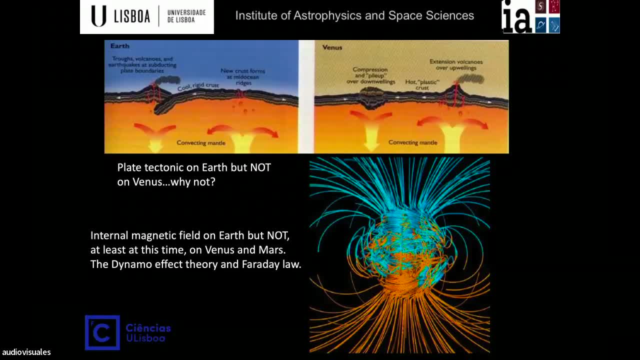 that we removed a lot of, a great deal of that. we removed a lot of, a great deal of co2 from the atmosphere on co2, from the atmosphere on co2, from the atmosphere on on venus, due to this process on earth on venus, due to this process on earth. 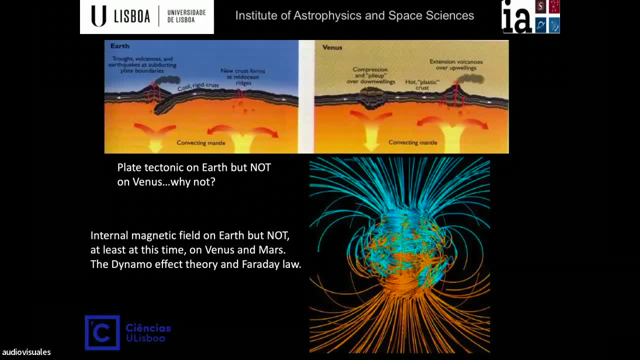 on venus due to this process on earth. so earth is the case that is utterly so. earth is the case that is utterly so. earth is the case that is utterly different from the other rocky planets, different from the other rocky planets, different from the other rocky planets. another thing that i want to: 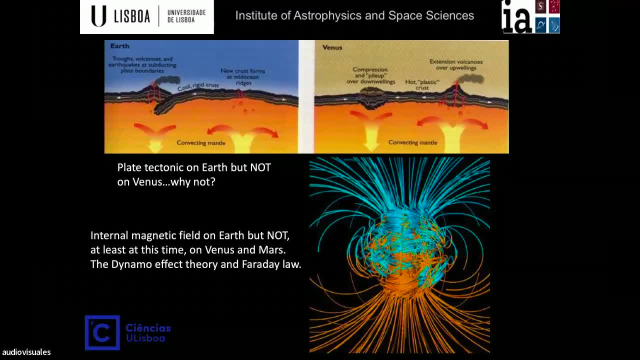 another thing that i want to, another thing that i want to to go deeper, but i don't know yet to go deeper, but i don't know yet to go deeper, but i don't know yet. we will try to address these questions. we will try to address these questions. 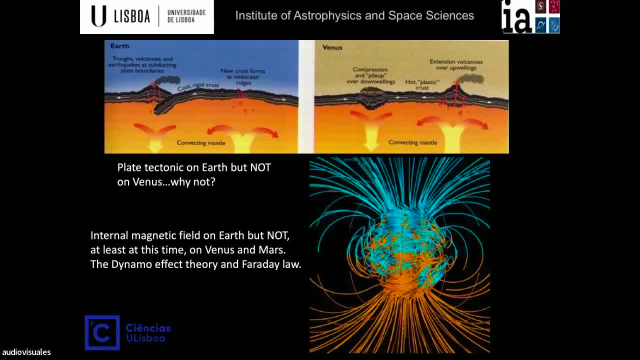 we will try to address these questions using the capabilities of the new space, using the capabilities of the new space, using the capabilities of the new space mission that is being prepared now and mission that is being prepared now and mission that is being prepared now. and vision, vision. 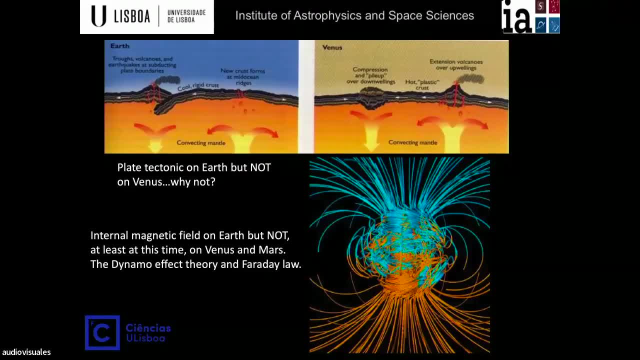 vision to uh to venus, that is to uh to venus, that is to uh to venus. that is the interaction between the subsurface, the interaction between the subsurface, the interaction between the subsurface and the and the and the lower layers of the atmosphere, of course. 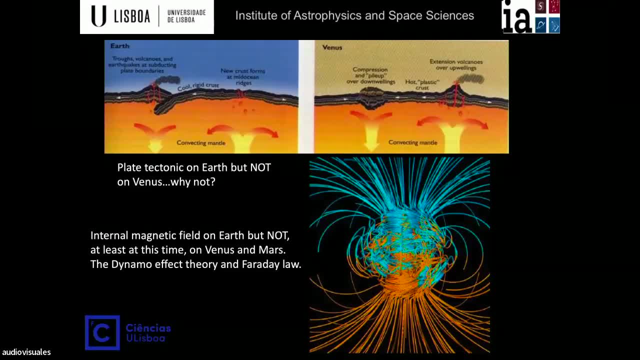 lower layers of the atmosphere? of course. lower layers of the atmosphere, of course, the so2, the so2, the so2 and the extra so2 and the source of the and the extra so2 and the source of the and the extra so2 and the source of the planet. replenishment of so2 on venus. but 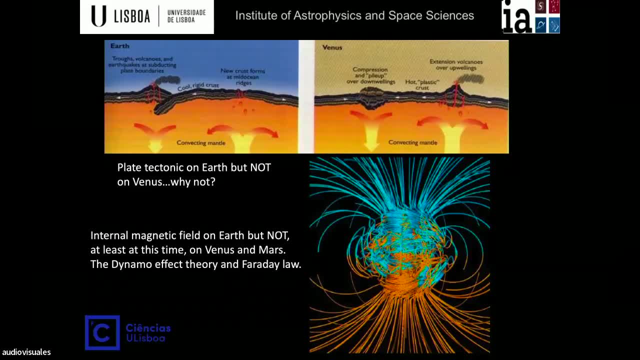 planet replenishment of so2 on venus. but planet replenishment of so2 on venus. but also also also, why it seems that on venus, why it seems that on venus the internal it is lower than on earth, the internal it is lower than on earth. 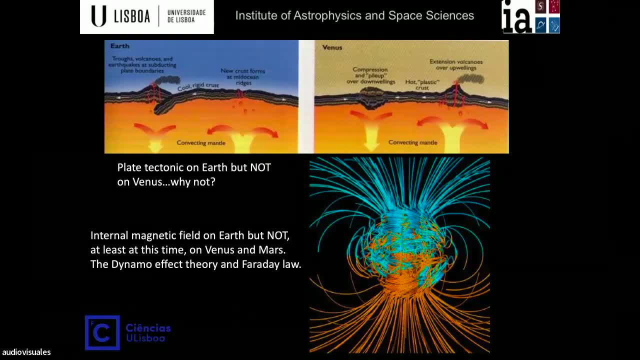 the internal. it is lower than on earth and, of course, the volcanism being and, of course, the volcanism being and, of course, the volcanism being different. we already explained different. we already explained different. we already explained it's connected with water. it's connected with water. 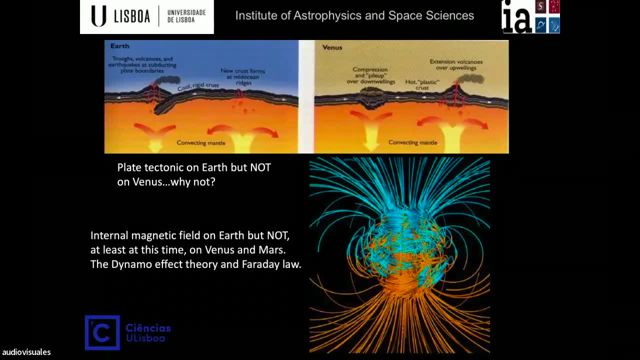 it's connected with water. i would say almost directly, i would say almost directly, i would say almost directly, of course, the timing being, of course, the timing being, of course, the timing being. this explanation is at the simple level, this explanation is at the simple level, this explanation is at the simple level, but i will start as i say, as i said, 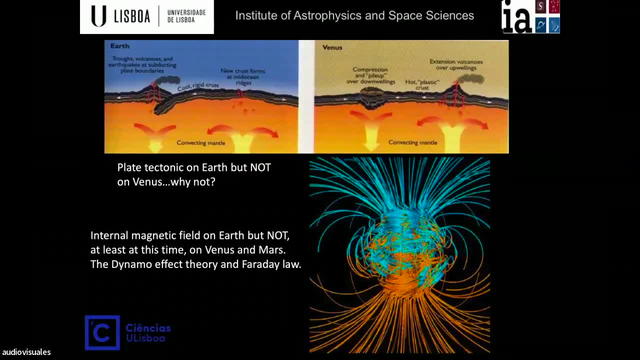 but i will start, as i say, as i said, but i will start, as i say, as i said, in this simple level. another thing, that in this simple level, another thing, that in this simple level, another thing that we must address to understand these. we must address to understand these. 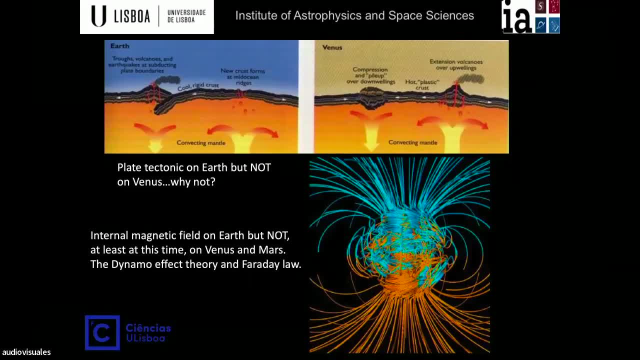 we must address to understand these different temporal evolution of the different temporal evolution of the different temporal evolution of the atmospheres in magnetic fields, atmospheres in magnetic fields, atmospheres in magnetic fields, and, and, and i was speaking a lot about venus, but i was speaking a lot about venus, but 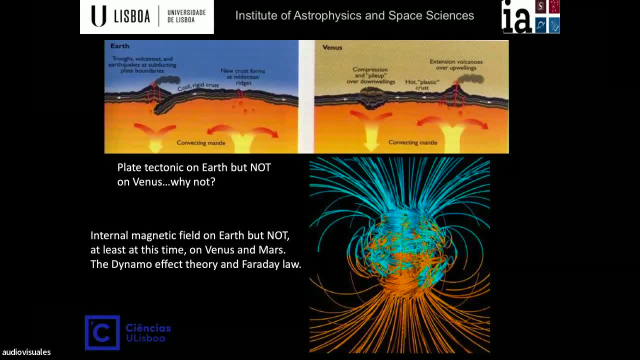 i was speaking a lot about venus, but let's, let's, let's give an eye to mars, give an eye to mars, give an eye to mars on mars, on mars, on mars, the, the, the. the atmosphere is the. the atmosphere is the. the atmosphere is much of much lower density than on. 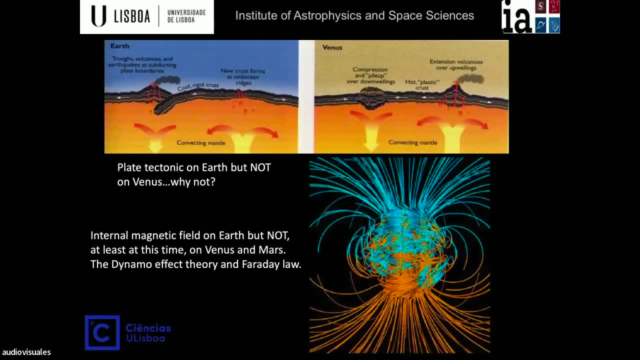 much of much lower density than on, much of much lower density than on earth. that we know earth, that we know earth, that we know that outcome, that outcome, that outcome, well, one thing is connected directly, well, one thing is connected directly. well, one thing is connected directly with the. 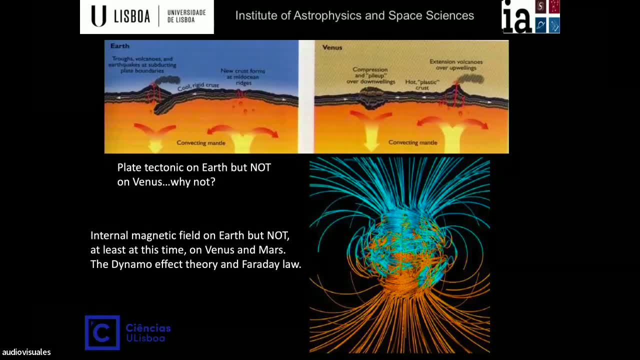 with the, with the, the mass of the planet, but i would say the mass of the planet, but i would say the mass of the planet, but i would say that that, that that's not direct, that's not direct, that's not direct, and we have, and we have. 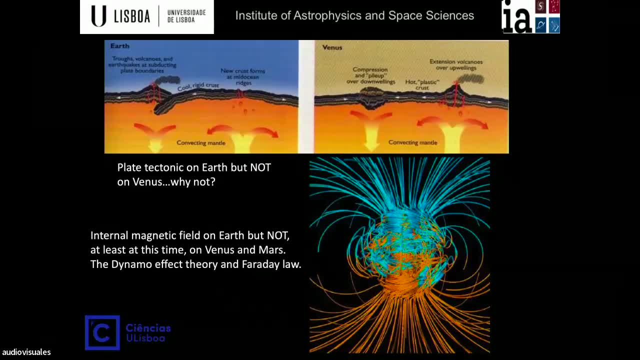 and we have a lot of evidence about higher density in a lot of evidence about higher density in a lot of evidence about higher density in the past on mars with water at the, the past on mars with water at the, the past on mars with water at the surface, and we all know that. but let's 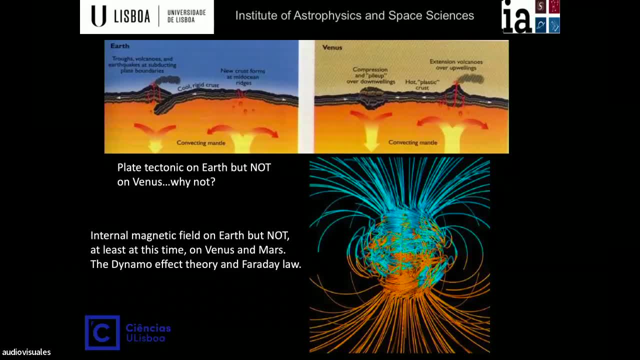 surface, and we all know that. but let's surface, and we all know that, but let's give an eye about, give an eye about give an eye about what produced this difference in the, what produced this difference in the, what produced this difference in the temporal evolution. and one thing is: 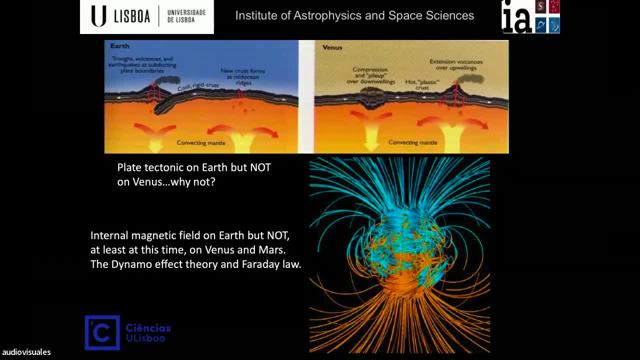 temporal evolution, and one thing is temporal evolution and one thing is connected with magnetic field, connected with magnetic field, connected with magnetic field. of course you know that. of course you know that, of course you know that the internal magnetic field on venus, the internal magnetic field on venus, 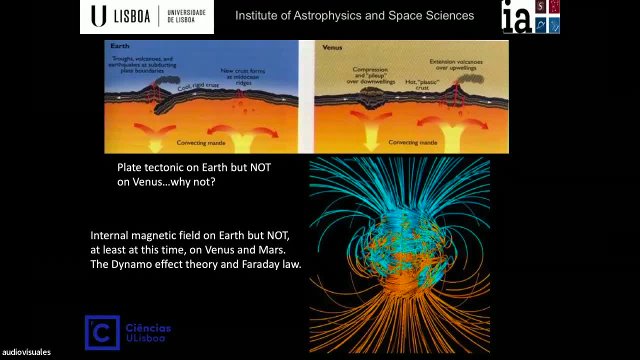 the internal magnetic field on venus? is there is no evidence? there is induced? is there is no evidence there is induced? is there is no evidence there is induced? magnetic field in the magnetic field in the magnetic field in the higher layers of the atmosphere, but not higher layers of the atmosphere, but not. 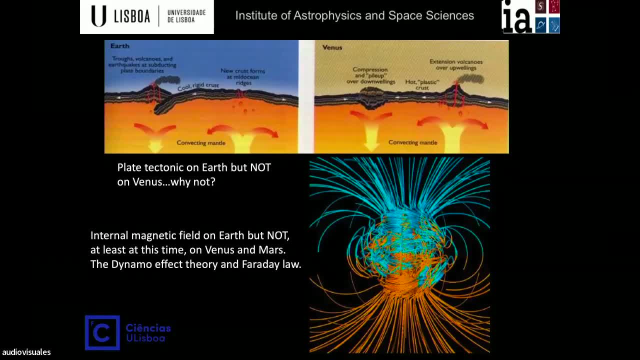 higher layers of the atmosphere, but not in the, in the, in the inner, inner, inner magnetic field. how come magnetic field? how come magnetic field? how come? very easy, very easy, very easy. venus rotates very slow. venus rotates very slow, venus rotates very slow, slow, even one year. slow, even one year. slow, even one year is is. is the length of one year. is the length of one year. is the length of one year is shorter than one day shorter than one day? shorter than one day: 2019: 219 to 2019: 219 to. 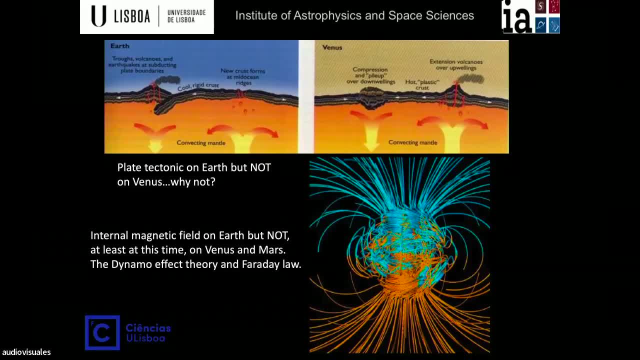 2019: 219 to 243 days. more or less 243 days. more or less 243 days. more or less so. so, so, as you see, it's not effective. the. as you see, it's not effective. the. as you see it's not effective. the rotation to produce by the dynamo. 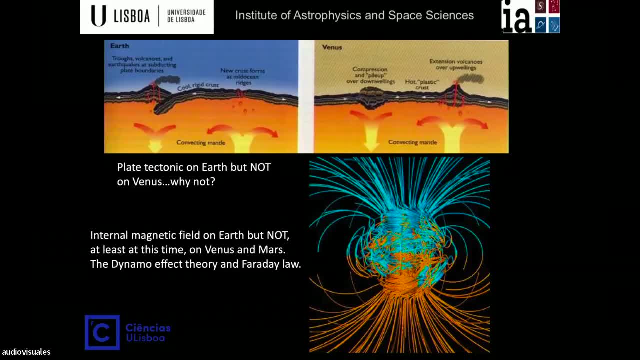 rotation to produce by the dynamo, rotation to produce by the dynamo effect by friday law, effect by friday law, effect by friday law. important magnetic, internal magnetic. important magnetic internal magnetic, important magnetic internal magnetic field, that's one thing. field, that's one thing. field, that's one thing. but what happens with mars? 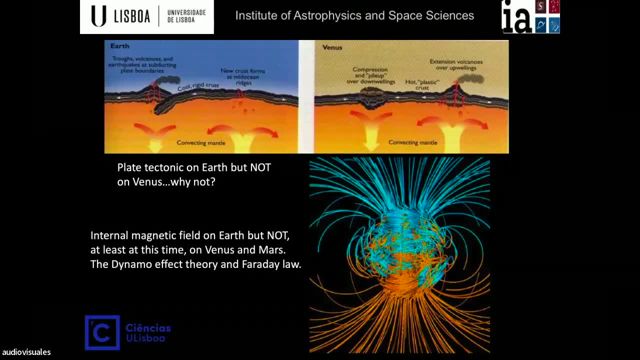 but what happens with mars? but what happens with mars? because mars rotates as earth by, because mars rotates as earth by, because mars rotates as earth by coincidence one day, coincidence one day. coincidence one day on mars is 24 hours. so this argument on mars is 24 hours, so this argument. 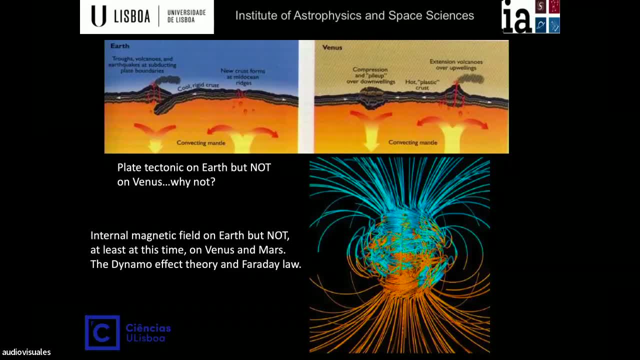 on mars is 24 hours, so this argument doesn't work, doesn't work, doesn't work, of course not, but of course not, but of course not, but a a, a roll bread, roll bread, roll bread will cool down, will cool down, will cool down much faster, much faster. 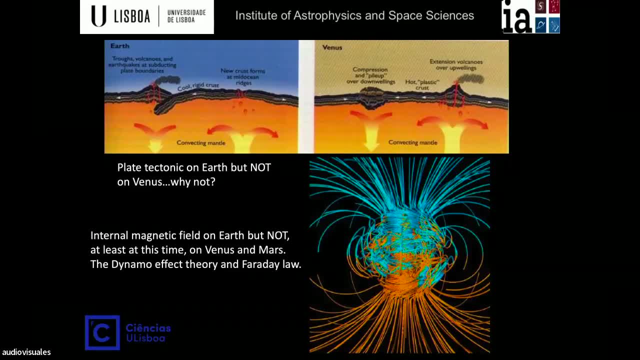 much faster than a huge bread. i used to. if i'm in than a huge bread i used to. if i'm in than a huge bread i used to. if i'm in portugal, i would say a power length. portugal, i would say a power length. 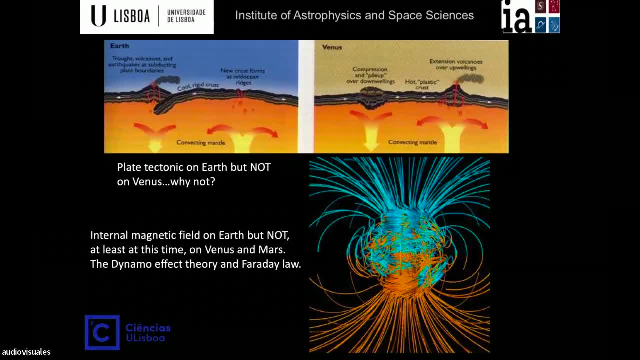 portugal. i would say a power length station bread from alentejo. that's a station bread from alentejo. that's a station bread from alentejo. that's a very big bread, very big bread, very big bread. here you please help me. what are the big? 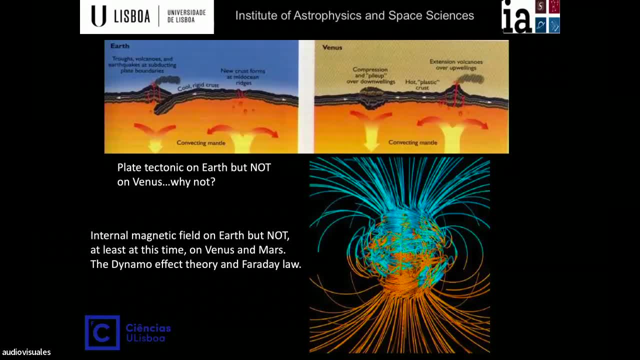 here you please help me. what are the big? here you please help me. what are the big breads in spain? breads in spain, breads in spain. so the thing is that the so. the thing is that the so. the thing is that the this, this is thermal conductivity. 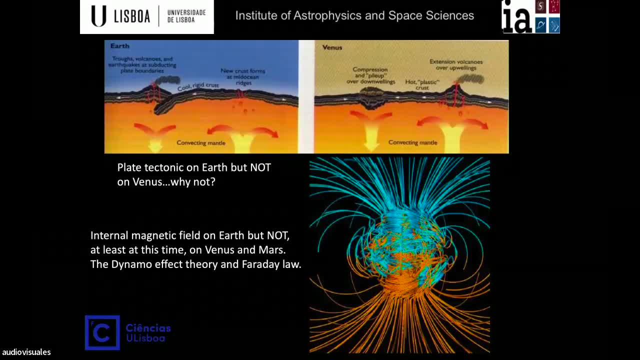 this, this is thermal conductivity. this, this is thermal conductivity. so it means that the small roll of so it means that the small roll of so it means that the small roll of bread with cooldown much faster bread with cooldown, much faster bread with cooldown, much faster than the big bread. 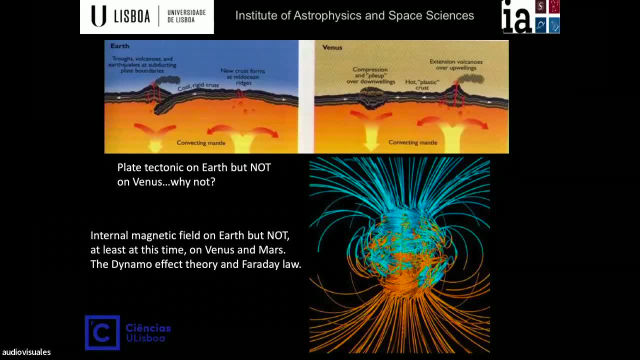 than the big bread, than the big bread. so, so, so, what i want to what i want, to what i want to do, the message that i want to pass, do the message that i want to pass, do the message that i want to pass with this, with this. 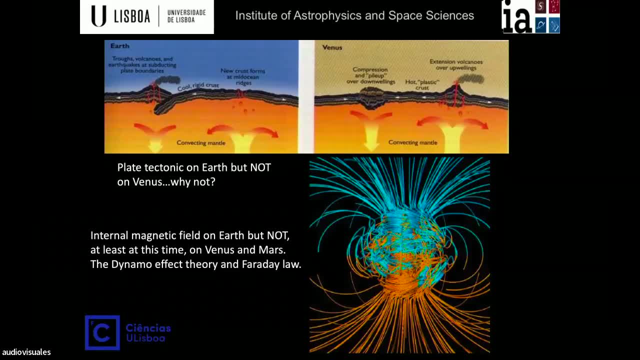 with this very awkward example is that mars. very awkward example is that mars very awkward example is that mars lost his inner. it's much faster than nurse. it's much faster than nurse. it's much faster than nurse, even if by for the dynamo effect, even if by for the dynamo effect. 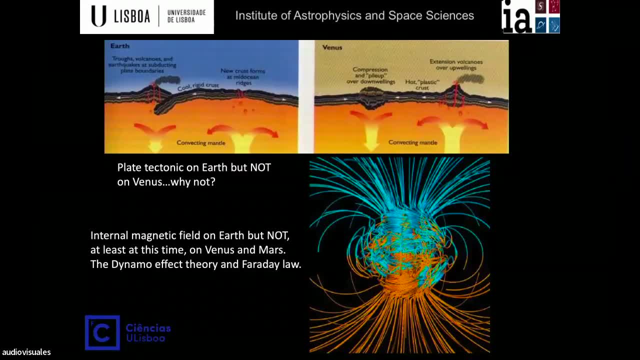 even if, by for the dynamo effect, it rotates, it rotates, it rotates fast enough, fast enough, fast enough. hazards at least, hazards at least, hazards at least, but, but. but the internal it, it's not enough. the internal it, it's not enough. the internal it, it's not enough to have enough. 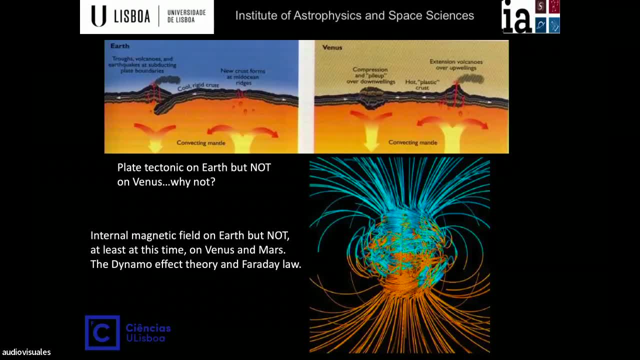 to have enough, to have enough ions and charges, ions and charges, ions and charges to produce, ions and charges to produce ions and charges to produce, by the farther law, this magnetic field, by the farther law, this magnetic field, by the farther law, this magnetic field, in a very effective way. 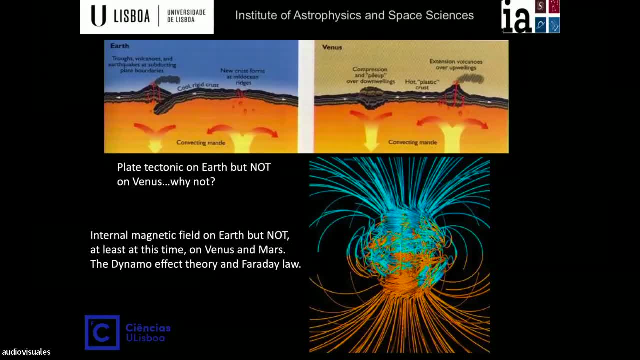 in a very effective way, in a very effective way. so the loss, so the loss, so the loss of these magnetic fields, perhaps in the of these magnetic fields, perhaps in the of these magnetic fields, perhaps in the past there were magnetic fields, even past. there were magnetic fields even. 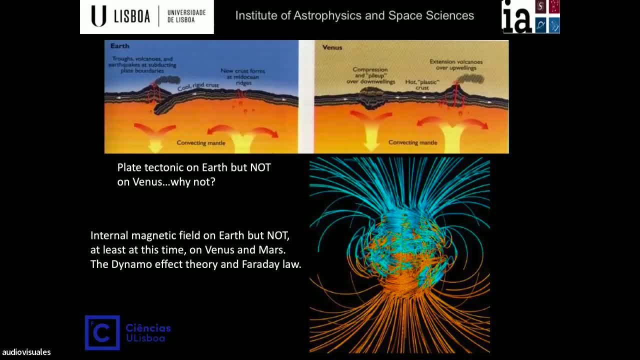 past there were magnetic fields, even relevant magnetic fields on mars. yes, relevant magnetic fields on mars. yes, relevant magnetic fields on mars. yes, there are, there are. there are some tiny evidence on that, of course, some tiny evidence on that, of course, some tiny evidence on that, of course that we must explore that better. 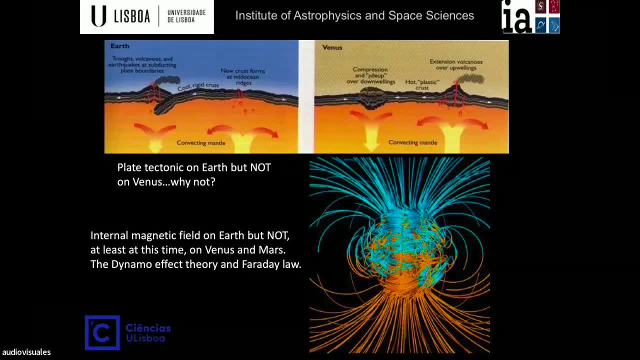 that we must explore that better, that we must explore that better. but i would say that we will find for. but i would say that we will find for, but i would say that we will find for sure. those laws of physics are always sure, those laws of physics are always. 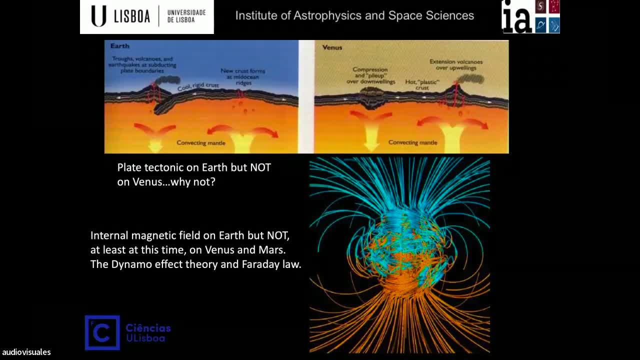 sure, those laws of physics are always the same besides the gravity law. that the same besides the gravity law. that the same besides the gravity law. that everyone knows that on monday morning, everyone knows that on monday morning, everyone knows that on monday morning the gravity law is much higher than the. 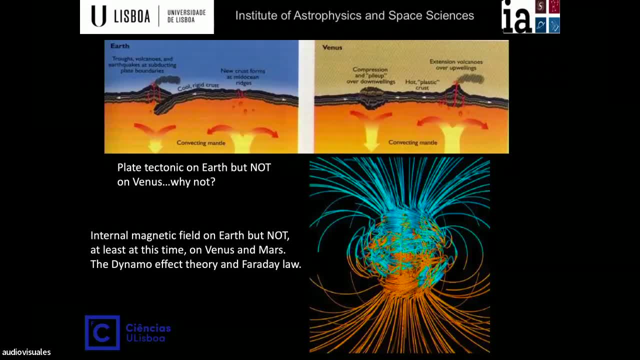 the gravity law is much higher than the. the gravity law is much higher than the common, but common, but common. but this is just a special case that happens. this is just a special case that happens. this is just a special case that happens on mondays. on mondays. 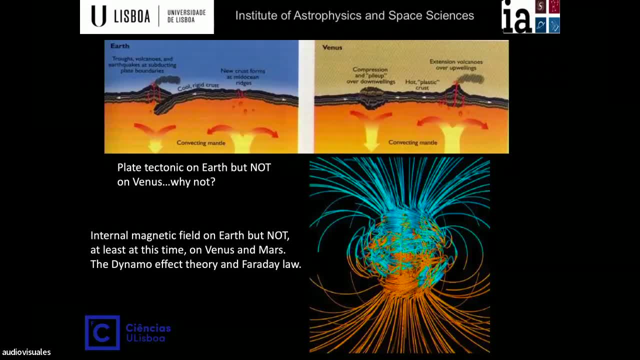 on mondays. besides that, besides that, besides that, the, the, the, the laws of physics are the laws of physics are the laws of physics are essentially the same, essentially the same, essentially the same. so again about what i was saying, so, so again about what i was saying so. 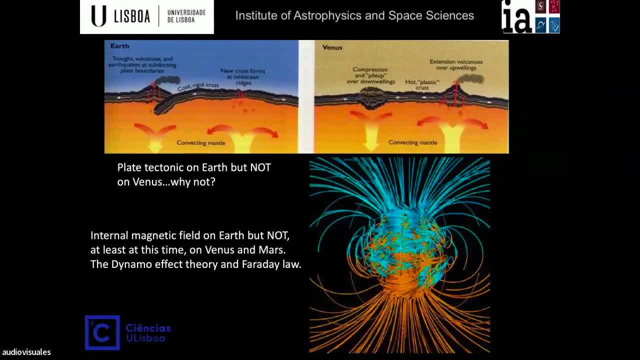 so again about what i was saying. so at time, at time, at time with time, with time, with time, and and, and. as outcome of this, as outcome of this, as outcome of this, we know by the, we know by the, we know by the, the, the, the diagram of phases by for water. 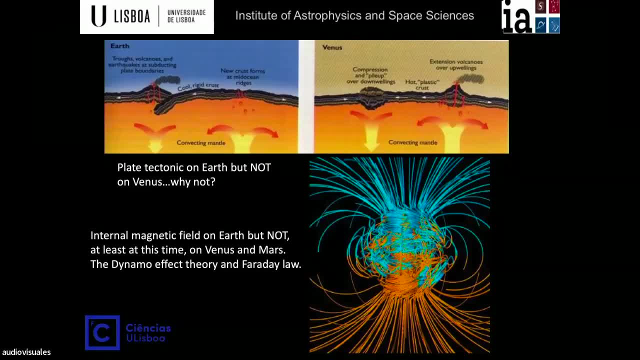 diagram of phases by for water. diagram of phases by: for water. due to the low pressure, and low due to the low pressure, and low due to the low pressure and low temperature at the surface, of course. temperature at the surface, of course. temperature at the surface, of course, connected with. 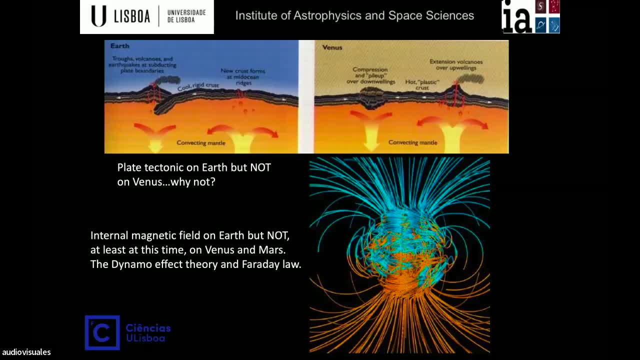 connected with. connected with not quite effective, not quite effective, not quite effective greenhouse effect. greenhouse effect: greenhouse effect today on mars. it means that it's not today on mars. it means that it's not today on mars. it means that it's not possible to have, possible to have. 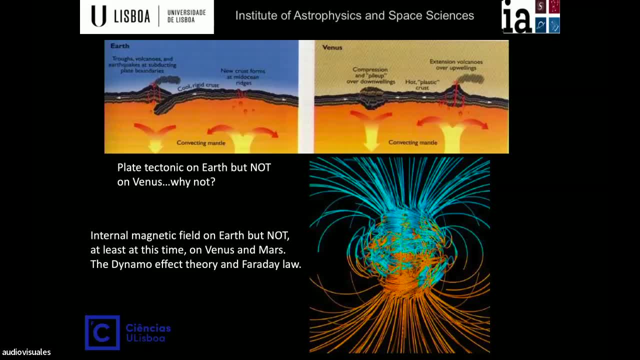 possible to have water in liquid phase at surface there. water in liquid phase at surface there. water in liquid phase at surface. there are some in the ghoulies, as you know on are some in the ghoulies, as you know on are some in the ghoulies, as you know on on spring. there are some. 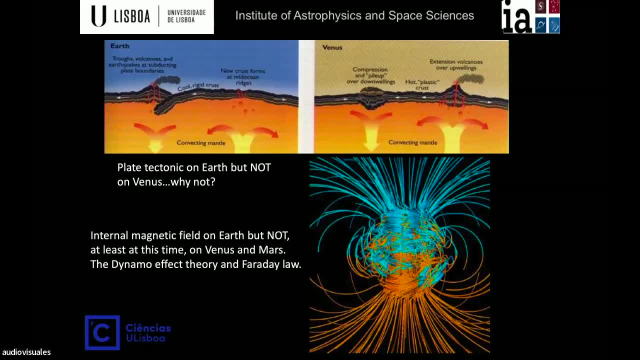 on spring. there are some on spring. there are some drops of water, drops of water, drops of water that arrives to the surface, mainly in that arrives to the surface, mainly in that arrives to the surface, mainly in the very steep, the very steep, the very steep craters, or 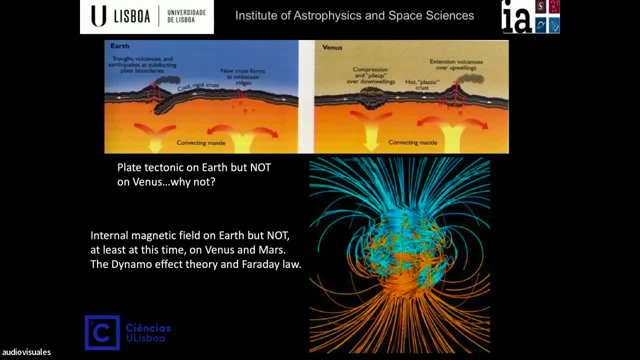 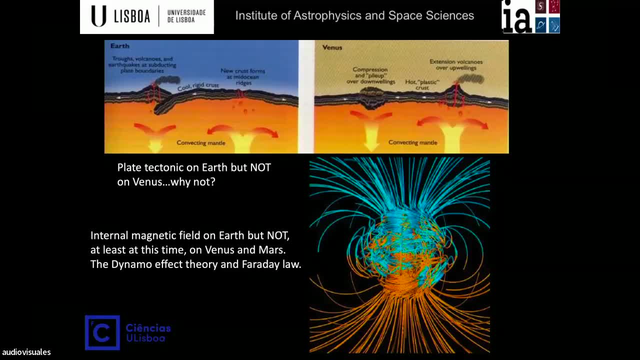 well in the liquid phase, because we well in the liquid phase, because we left some in the ices in the winter, left some in the ices in the winter, left some in the ices in the winter, hemisphere, as you know, hemisphere as you know, hemisphere, as you know. so, 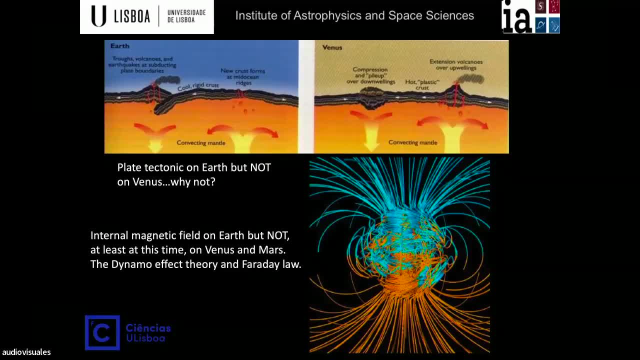 so. so this is a, this is a, this is a mostly a context for what i want to, mostly a context for what i want to, mostly a context for what i want to share with you about our share with you, about our share with you, about our research. 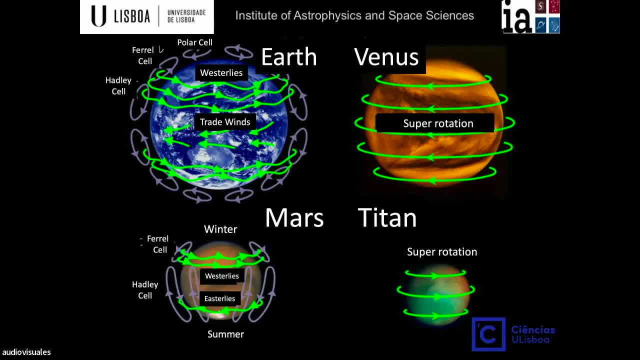 research, research. first one thing, that first one thing, that first one thing that is connected with these rotations and is connected with these rotations and is connected with these rotations and the fast rotators that are on the, the fast rotators that are on the, the fast rotators that are on the, on the, on the. 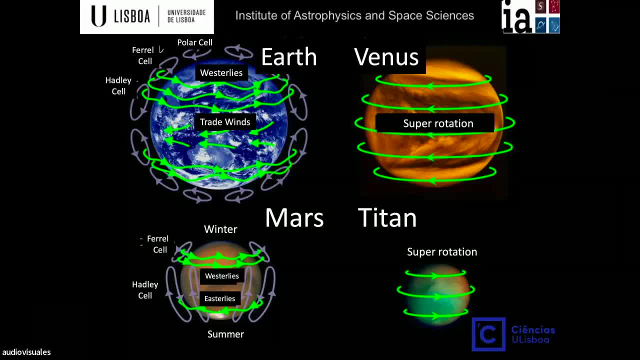 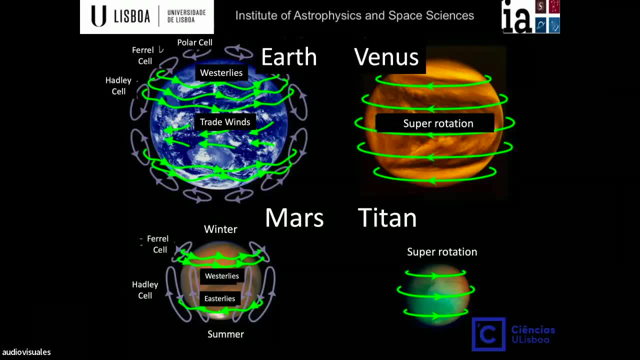 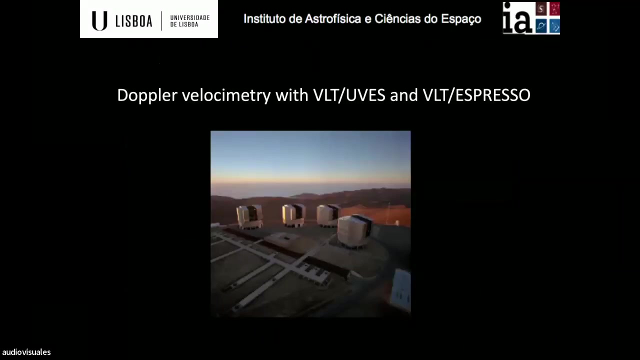 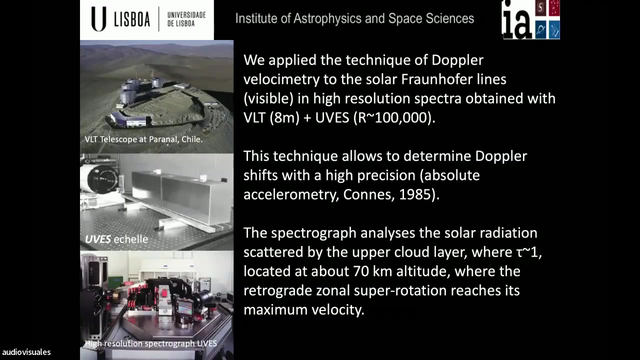 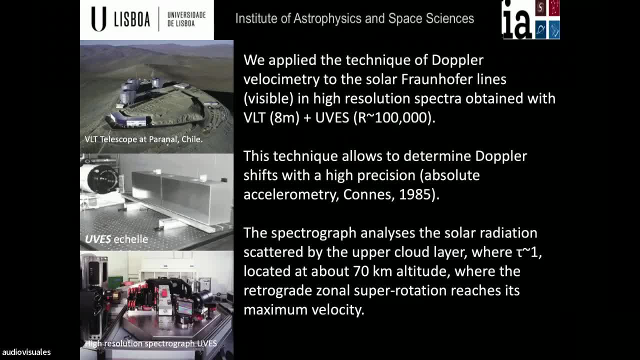 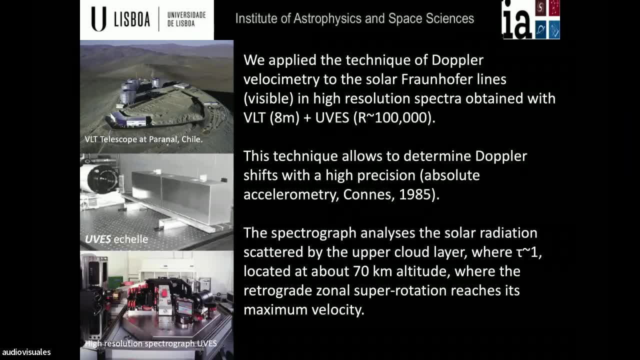 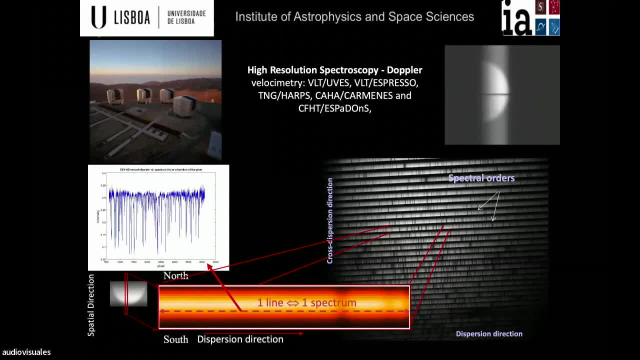 tracking from spacecraft, from space, from orbiters And from there. so this is one of the the raw data reduction that we do from the shallow grams, So from the basic data, till obtaining the 1d spectra. but they are high resolution, So at the same. 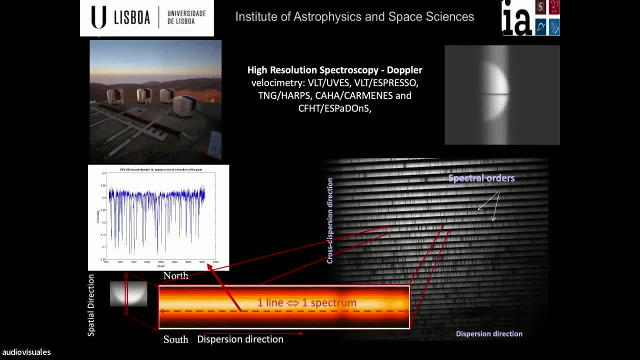 time we can produce dynamics and we saw we can go for is a topic ratios, because we have extremely high spectral resolution and also study minor components, And this will be the second part of this talk. So we start with dynamics And so we 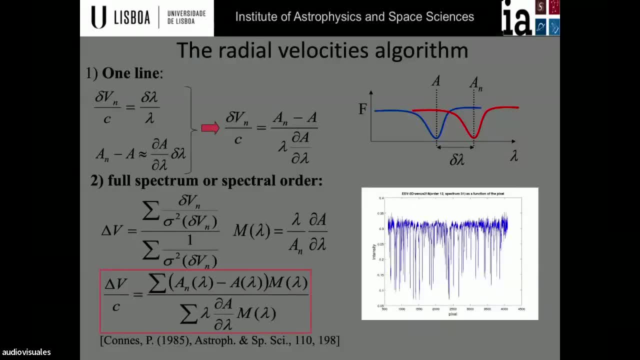 could take the most from our data. of course, and we this too- much equations before lunch, But this is very easy. What I want to show here is: from the shift of just one line is impossible, impossible to retrieve With the, with the precision we need about five to. 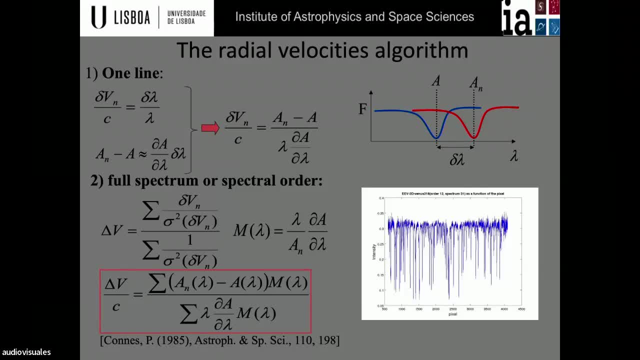 10 meters per second in precision, the velocity of the winds, for instance. So what we do is, in fact, is what is in this, In this system of equations? here we perform a wafered average using all the front of the lines. 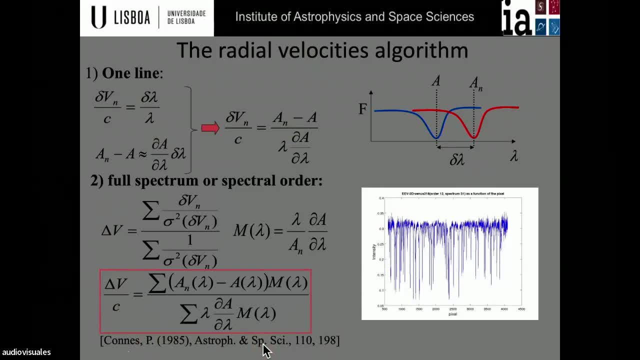 about 4400 lines, all the shifts, using as a weighting coefficient in the inverse of the variance related to each, each line. With all this statistic, we can measure the winds with an error that can go for, for instance, VLT Espresso with about one to. 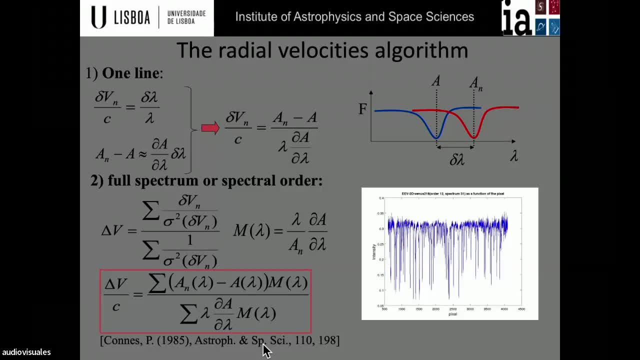 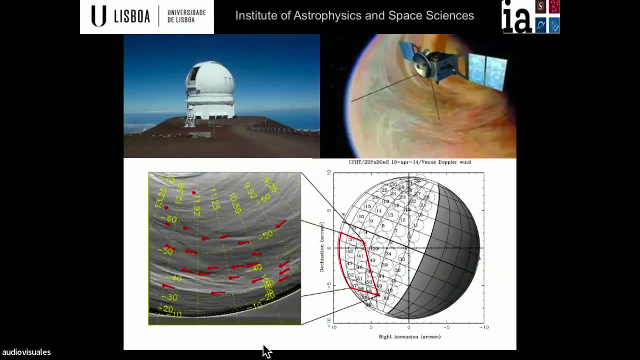 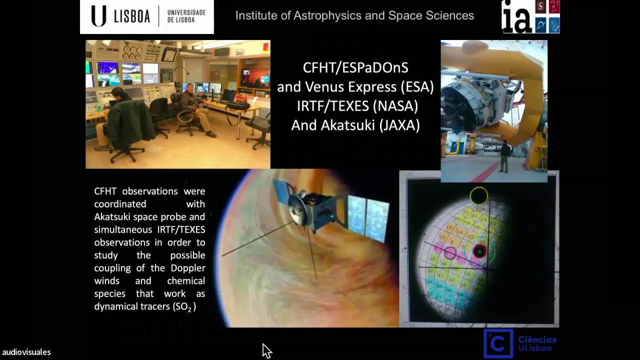 two meters per second from ground based observations. That's incredible. So at the same time, as I said, we perform coordinated observations. This was in the past with the, with Venice Express. Now we use Akatsuki in order to perform this kind of studies. but I will not take too much time on here. The 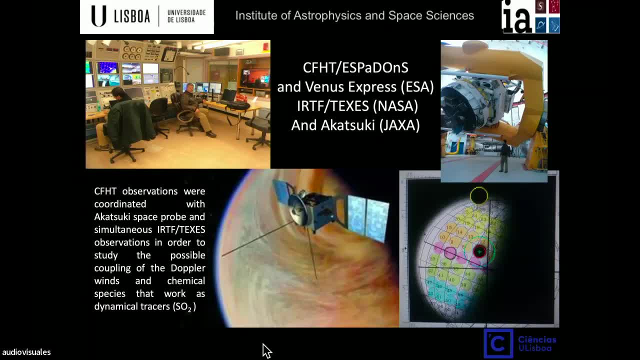 only thing that I want to share with you here, that is, in these observations. we were observing, observing coordinated with IRTF Texas, with Tejas and Khana from Paris Observatory, in order to retrieve the SO2 in the presence of and variability of the SO2,. 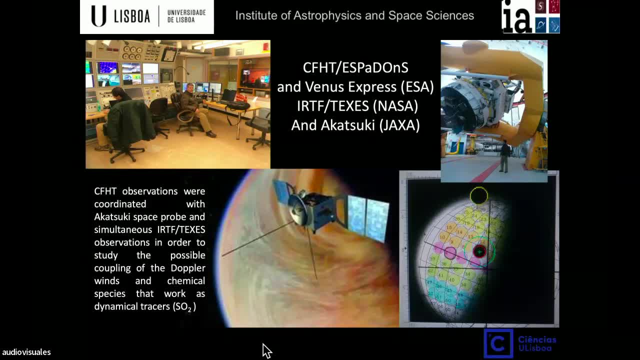 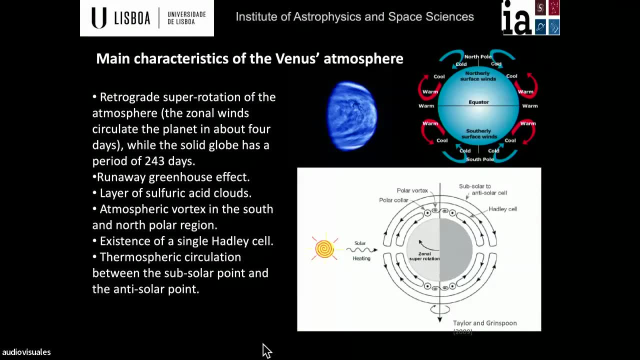 the temporal and spatial variability of the SO2. And that was quite important at the time. So some basic stuff about the atmosphere of Venus. I think that I will not go too deep on this. Most of the things that I wanted to pinpoint to you I. 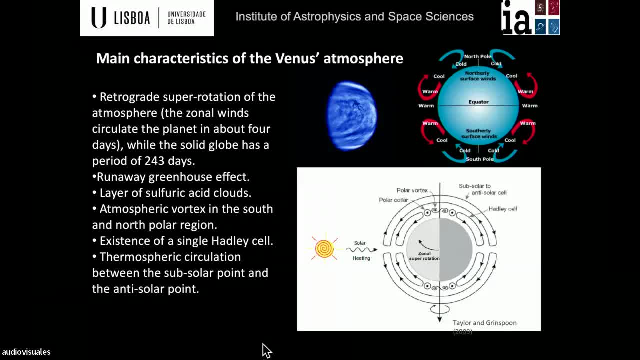 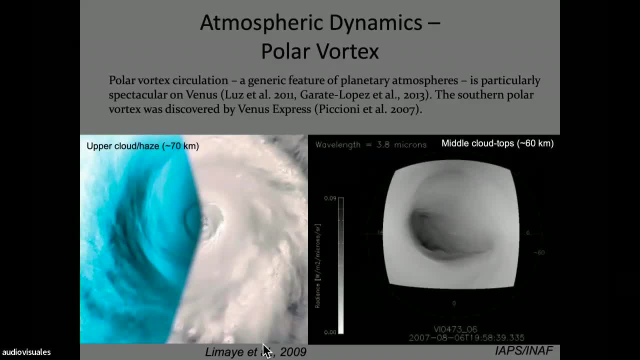 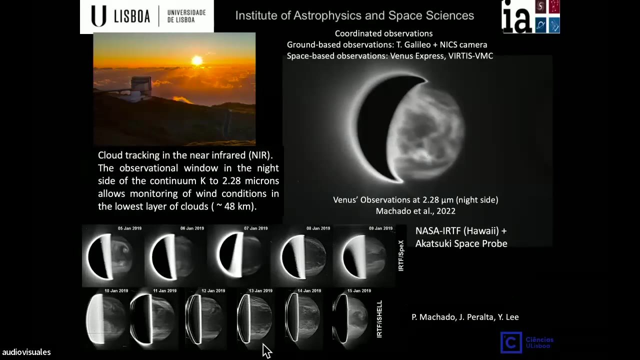 already said. So the rest, if there is any question, I will be happy to answer. So we also use the cloud tracking from the space probes, for instance, to study the vortex that is highly variable on Venus at the time. And from here I want also to 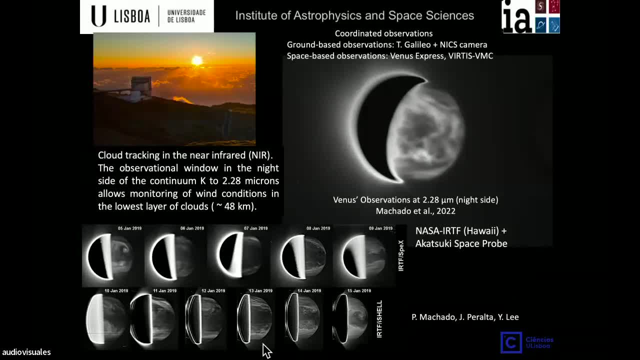 share that we have this relevance of studying the same dynamics from space. And well, there are some tricky things, like, for instance, that was the first hurricane on Venus detected in our observations, and with a Spanish friend and collaborator, Xavier Peralta, And what I 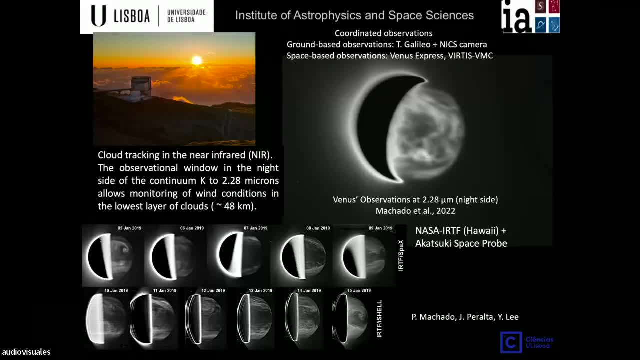 want to say is: in our observations we started to detect a lot of atmospheric gravity waves And this could be very important to trigger, to accelerate the horizontal layers of the atmosphere in this phenomena of the super rotation of the atmosphere that we have evidence on on Venus. 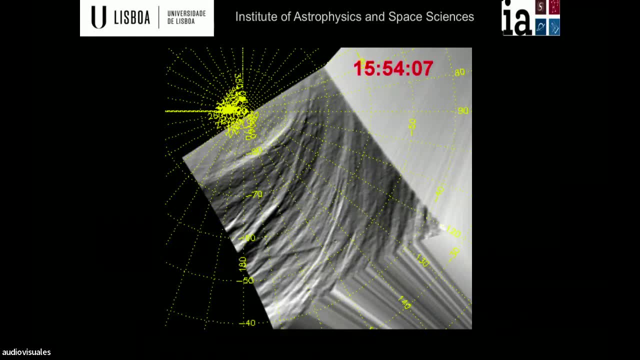 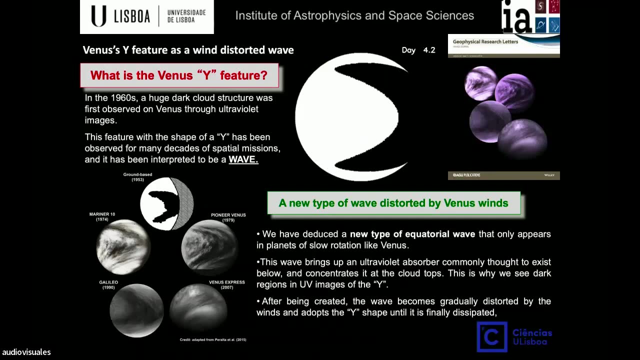 So this is the basis of the cloud tracking. of course it moves with time and well, I will not go also in very deep on this, but we were interested in studying the, the atmospheric waves. these are planetary scale waves, the y-shaped wave- that for more than 60 years, 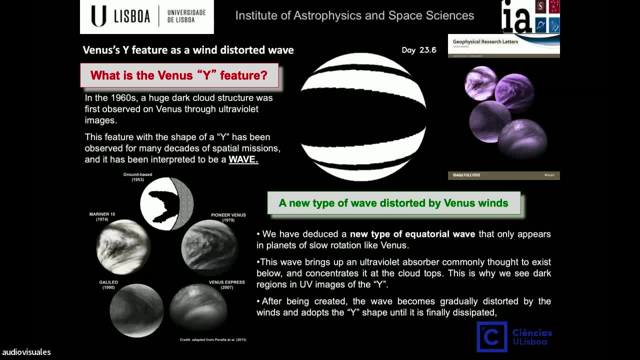 we couldn't understand, and this is a caution, even if I totally 100% go to modeling. modeling is very important, helps me a lot in in our observations and so it's a we in relation with modeling. so I support 100% modeling, but we must be careful. and one thing: 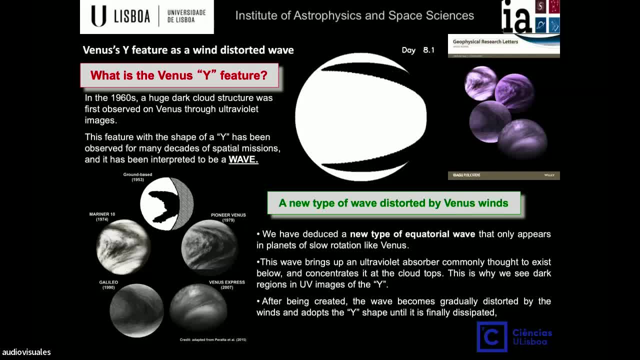 is why, and the basis of this work that is related to it, something that we we departed from the model of Earth because Earth observers, they have the terabytes. of course that we have the extreme cases, but they have the terabytes. so we started from Earth model and adapted to. 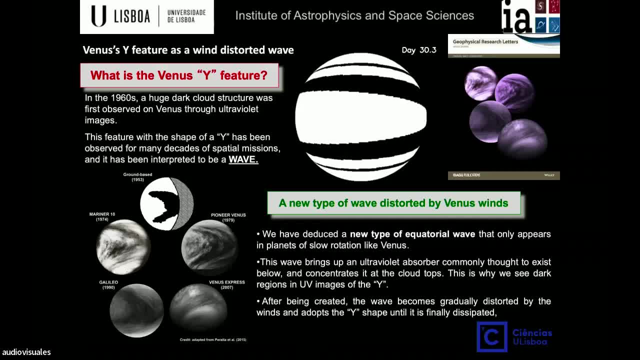 Venus, And we couldn't. we couldn't model this y-shaped wave, so what we did was to vanish everything we know and started from the scratch, from the primitive equations and from the basic equations and from the differential equations related with dynamics, and from there we could, in our model, nicely predict. 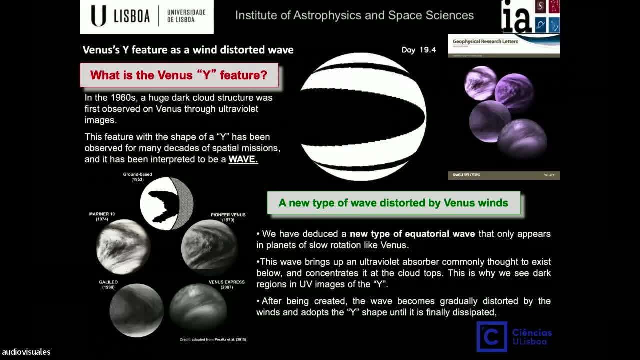 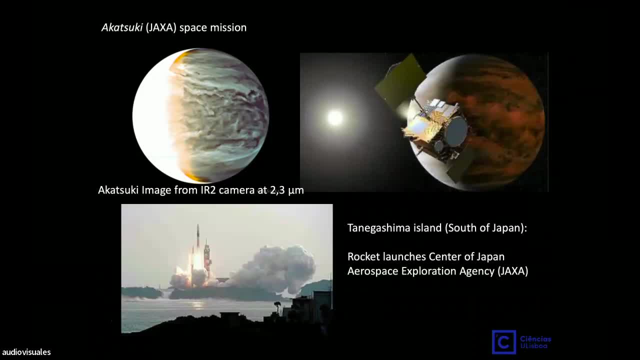 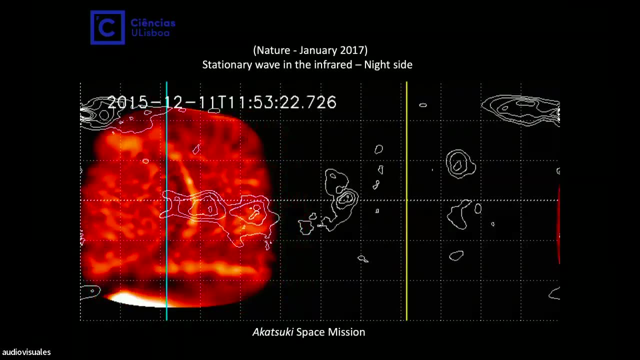 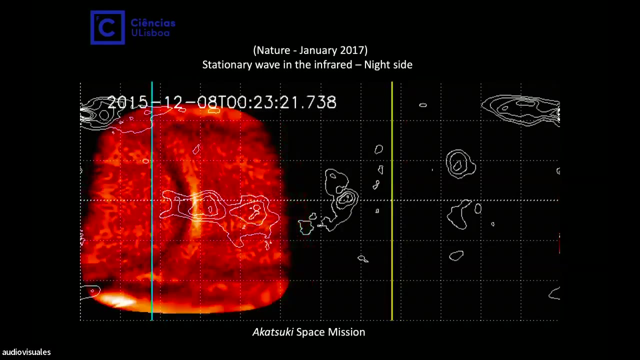 the shape of the waves into the y-shaped wave, as you can see. So now we use Akatsuki, and that is the only orbiter that is in the orbit of Venus at this time, and we were also interested in studying planetary scales, planetary scale waves, in this case in the 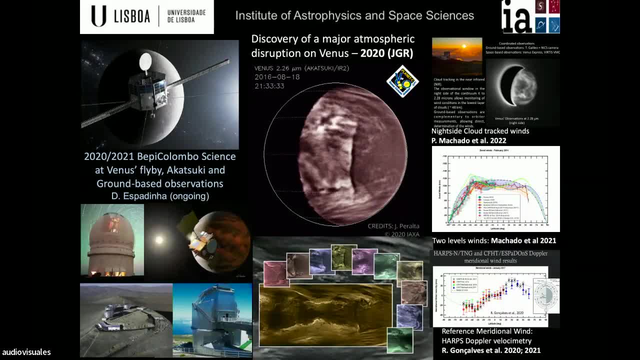 infrared. but from there we wanted to go deeper and to start to study planetary scales. So we go, go study lower layers of the atmosphere, like in that case that you can see there that is a huge disruption in the Venus atmosphere, like a huge frontal surface on the atmosphere, like a wall. 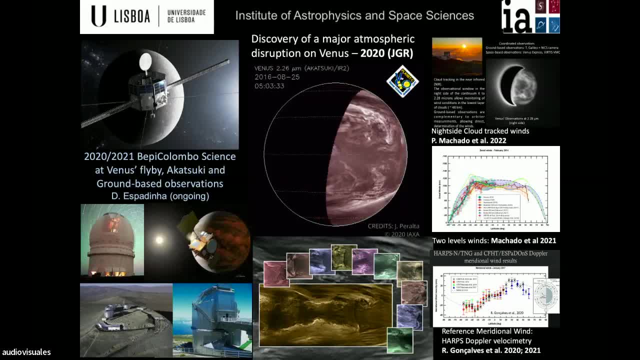 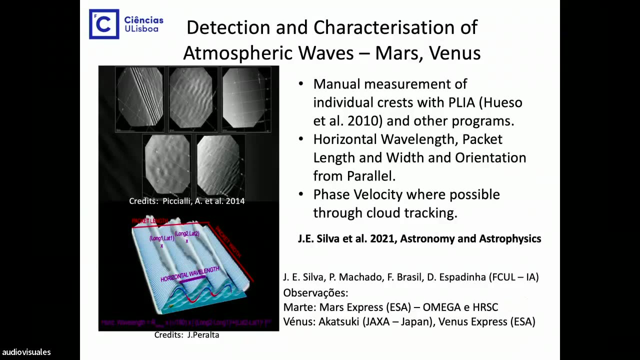 that could be very important for chemistry and related with something that I will discuss with you now about this case, about phosphine on Venus. Do you believe in that? So let's address this on the following: and we started also to study the mesoscale and minus. 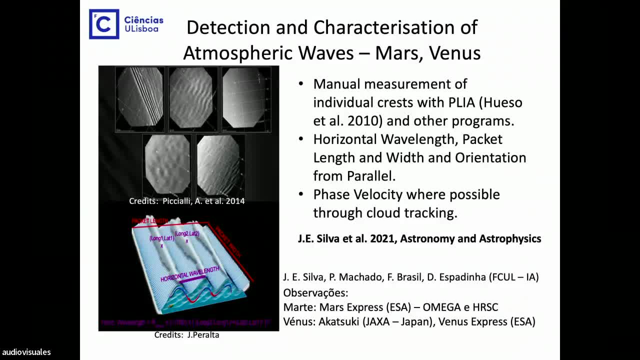 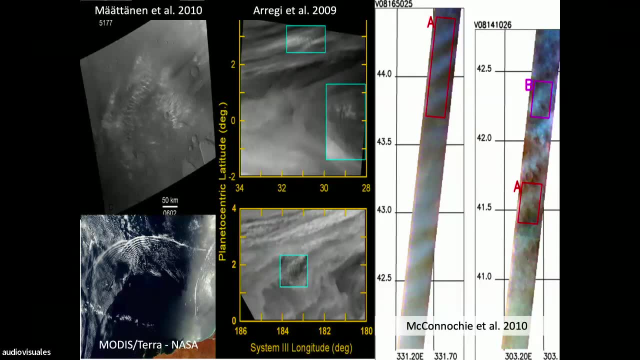 and minor scale waves on Venus and Mars using different techniques that we developed and fine-tuned and from that we started to first detect and, second step, characterize these waves Even could develop. now- it was last month- a method to measure the with precision, the altitude of the waves on Mars, because on Venus was very easy. 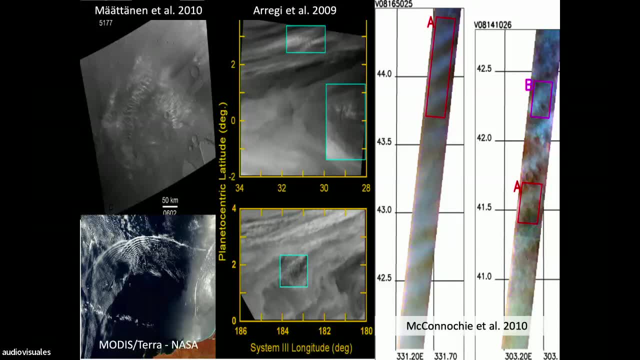 that was easy because we are on the shoulders of giants that studied that before. of course, that on Mars was not easy at all, but now we can do it. so that's very important to characterize the atmospheric gravity waves on Mars. and we can do it, that today. yes, we can. 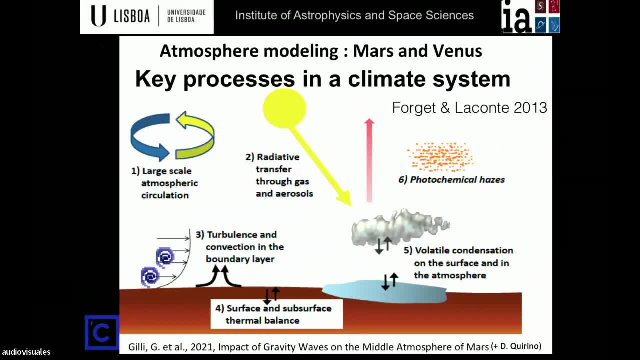 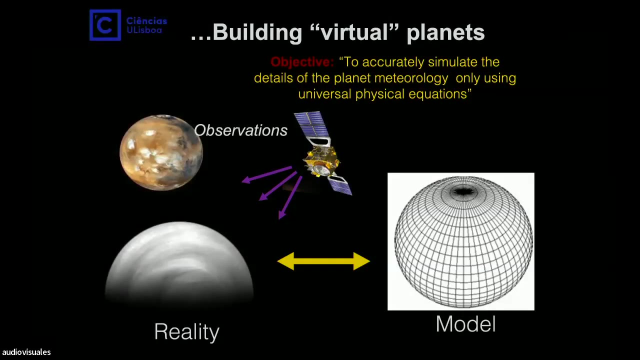 and, of course, related with model, always related to each model, with LMD on on the models from France, but also with models from Japan. so we are in close connection, collaboration with these two groups in order to fine-tune and connect the synergy between observations and modeling. and so it's what I'm saying. that is very important, but I want to go. 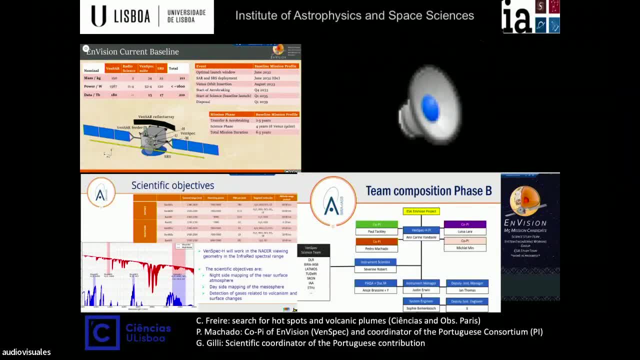 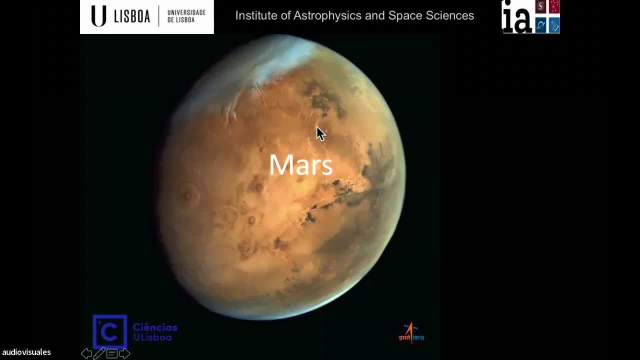 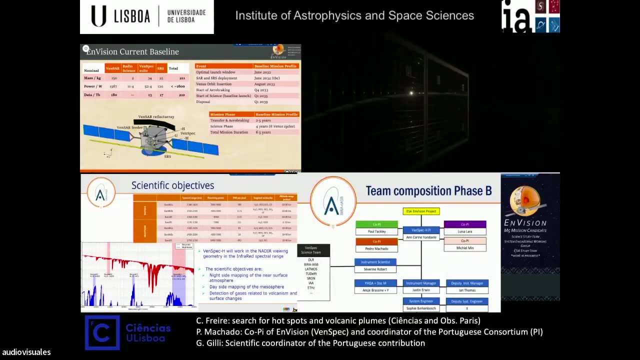 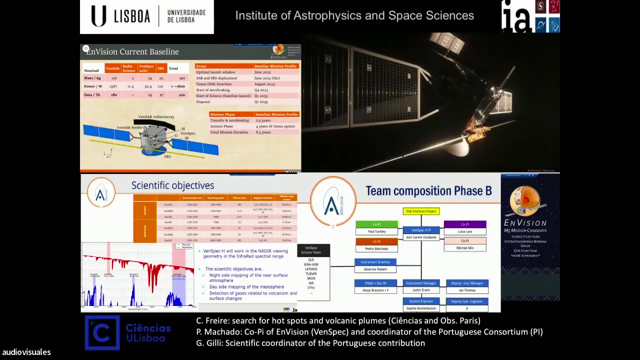 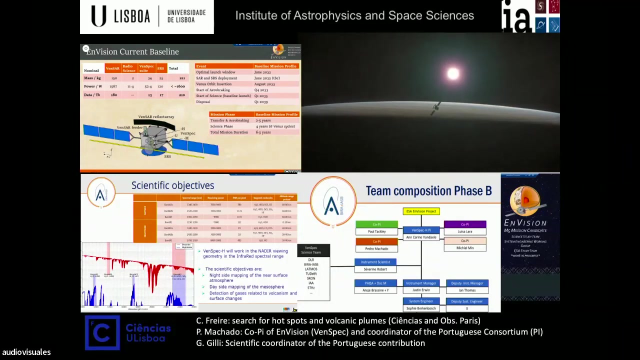 directly to the main things that I want to to to share with you. so this is related. this slide is related with Envision and Envision. because Venus is totally shrouded by clouds of sulfuric acid, it's difficult to map the surface and study the relation between the surface and the, the atmosphere and the replenishment as 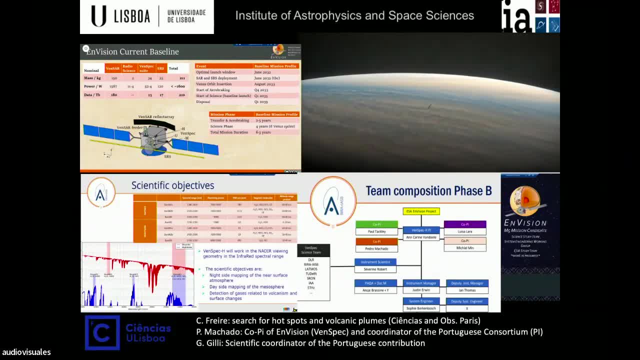 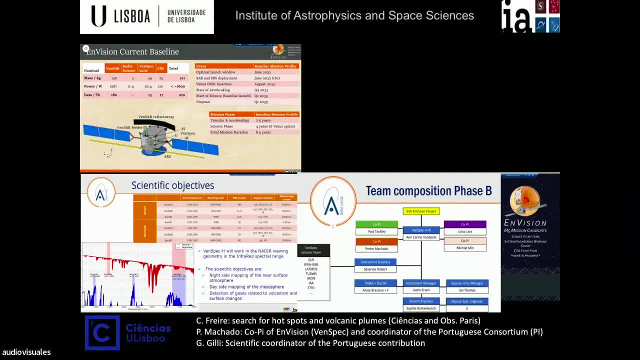 I said of the SO2, but also, are there vulcans on Venus? are they active? we are addressing that now. we are, and we are doing this study in a two-fold approach: first, looking to thermographic maps of the surface and to look for hot spots. 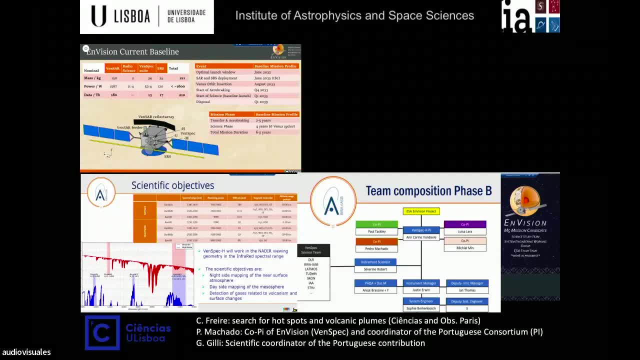 the first study was made with virtish, an instrument on venice express. now we are readdressing, reanalyzing this data from all the old mission. but also one thing that is important is the minor, minor cases like CEO, like HCN and other important cases related with you, with astrobiology. 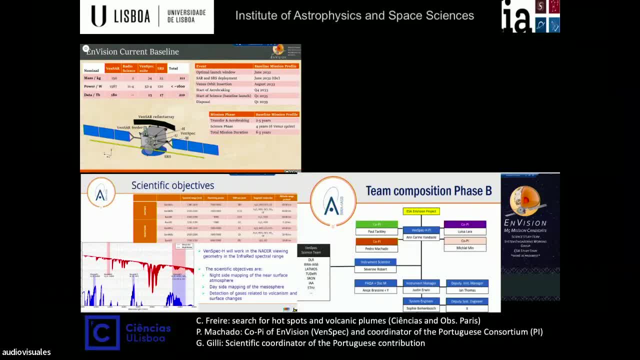 and we are in the process of detection, but it's not easy. so I hope that we can do it before the launch of Envision, otherwise we must wait a lot from the launch. but we are doing some work on that right now and we already had some close-up of the Venetianx and people-to-body対処, Vaudeville and the nnini. you can do some satellite. my code were going about in the domain, but we are already having additional elements, like we have already that various datasets that we are developing, doenerな, HCN and other important cases related to it. you with astrobiology, and we are in the process. 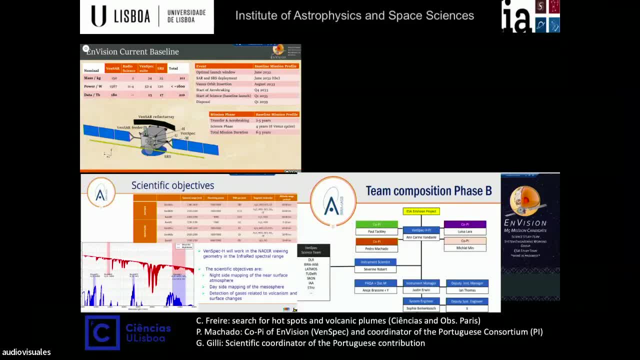 but is not easy. so I hope that we can do it before the launch of Envision, otherwise we must wait a lot from the launch. but we are doing some work on that right now and we already had some positive detections of some minor compounds on the atmosphere of Venus. but 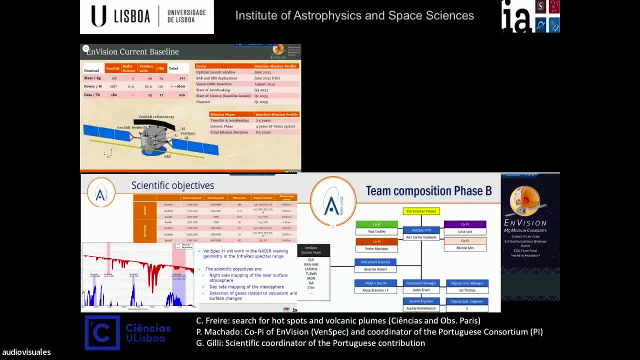 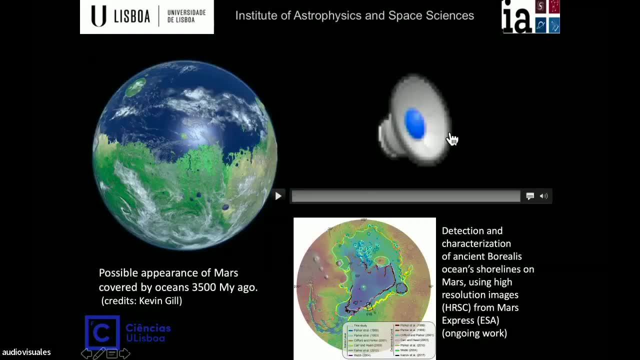 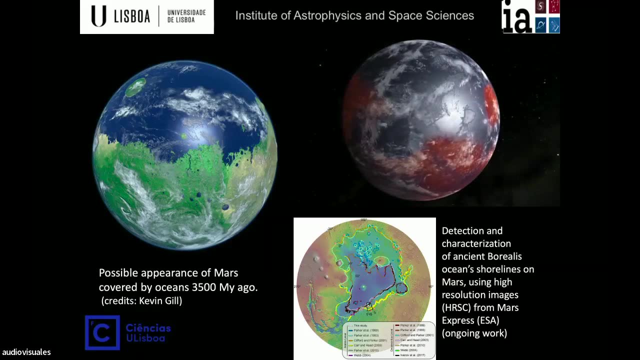 well, let's see in the paper that will come out, hopefully, in the next month. So now on Mars. you know about ocean borealis, of course, and that with time, that Mars lost most of its water. were there life on Mars? We don't know. There is Life on Mars. today is possible and we want to. 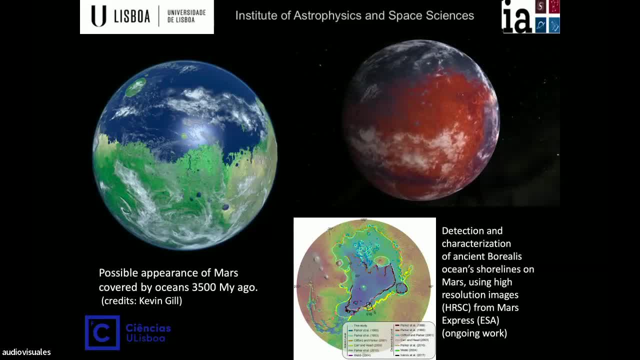 participate and collaborate in this huge task that is to perform this kind of investigation. It's, I would say, a marvelous adventure to look for this. and we, what are we doing? We are, in one way, we are portraying uh, ocean, ocean, cold shorelines and also fluvial marine systems on on on Mars, but not just at the 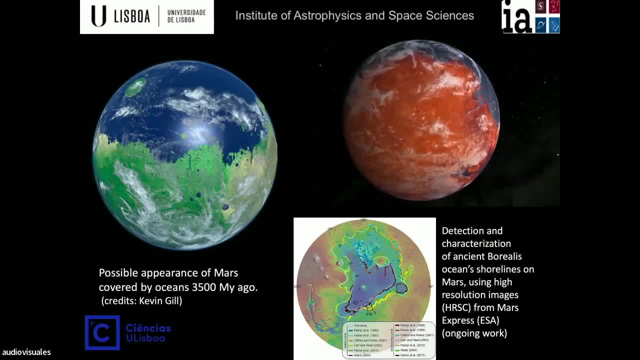 topographic level approach, but also uh, using uh omg instrument from Mars express uh we and using reflectance, we want to study the characterization of the minerals connected with these fluvial marine systems on Mars. That's it, Thank you. The next slide. 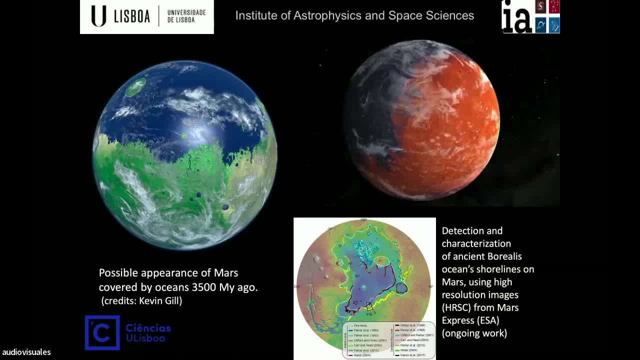 One of the things. that is one thing. the other thing is that in our small team we have connection with ExoMars, TGO- mostly Nomad instrument- but also with Mars express, mostly Omega instrument, that is, an image spectrometer- but also with the high 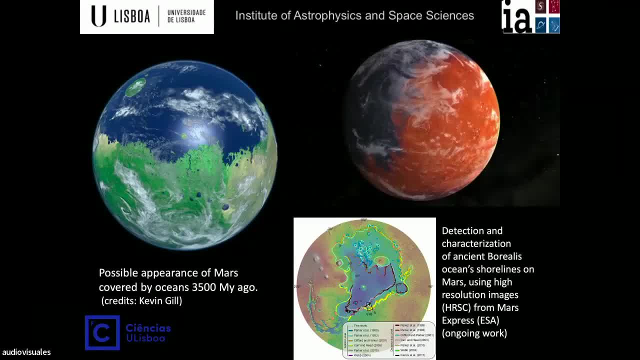 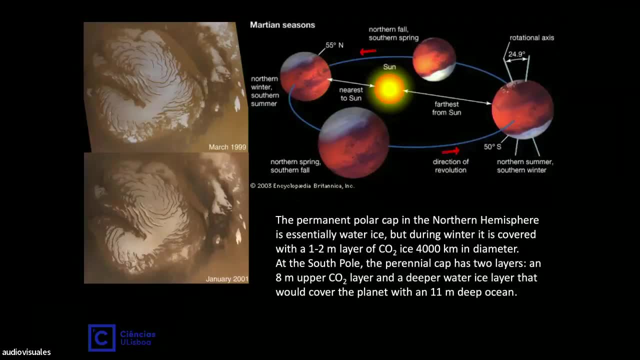 resolution camera, HRSC, Mars, and we are doing already is the characterization of the, the atmospheric gravity waves, but also about the methane. I will show you in a couple of slides. so that is the basic. so you know that there is enough water on on Mars, we know, and on on the. I already said about the surface, so I will skip this. 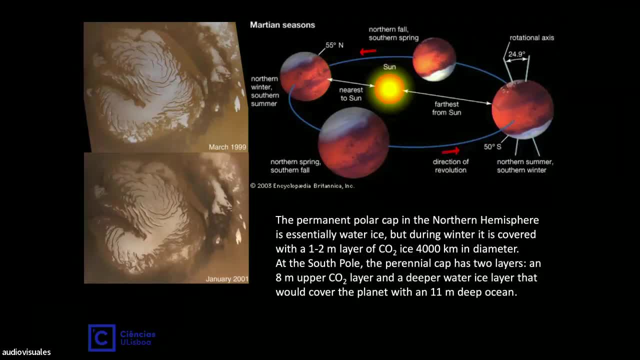 but, for instance, Mars Express detected huge reservoir Reservatories of water underneath the surface, uh, and there are recent evidence of uh water near equator and this is very important. this is very important that we add water. plus, time is important for life and if we add water, 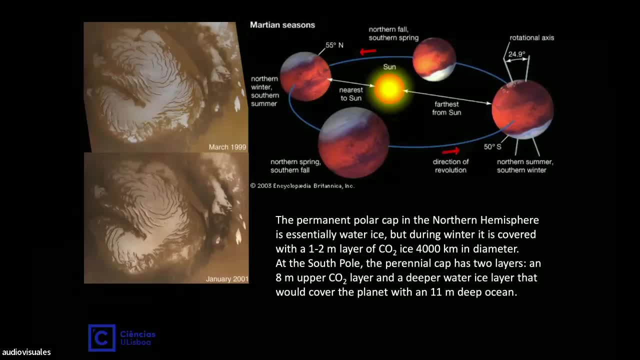 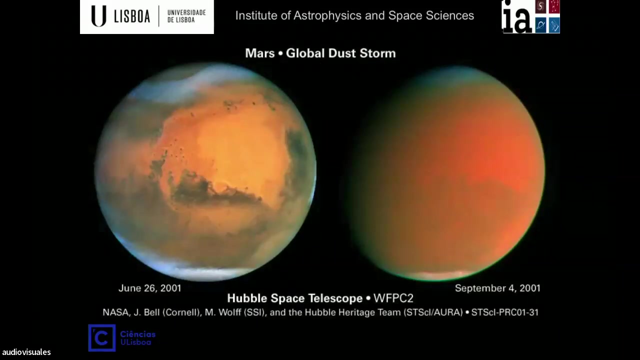 in the equatorial region for a longer time, mostly in the basins, in some sectors like G0 and others that are now on full study, as you know. that could be very interesting. uh, so one thing that affects very much the climate on on Venus, on Mars, sorry, is the dust storm that. 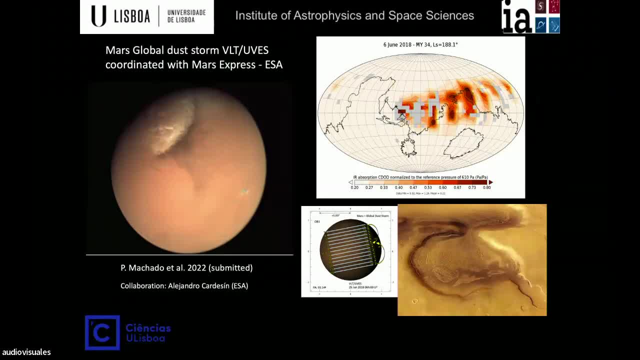 would be global. and this one thing that, uh, myself I'm studying with the same technique of the Doppler velocimetry. so measure winds on Mars is very difficult, really difficult, because it's so tenuous the atmosphere, but along even original the stone. with this technique we proved that we can retrieve and 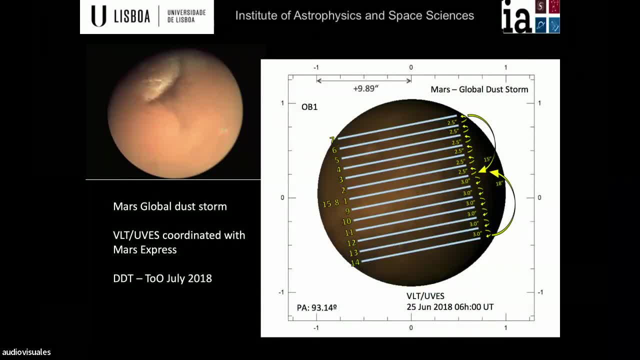 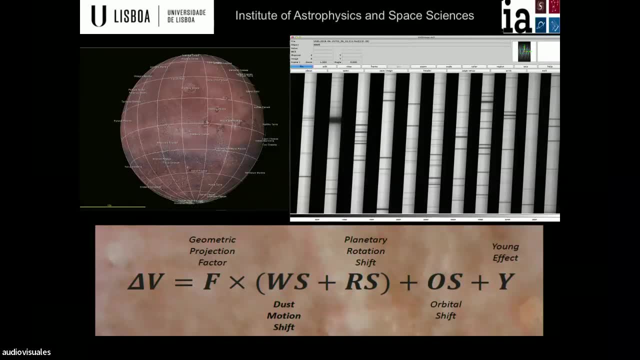 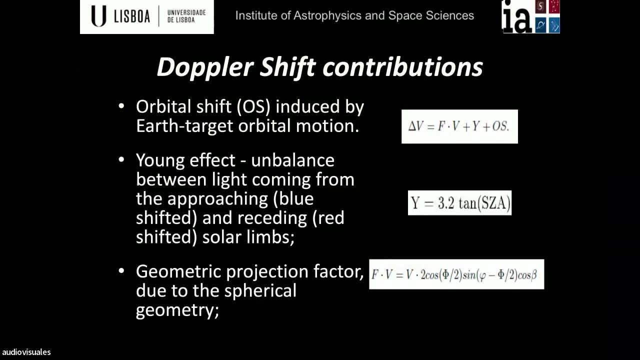 map the winds on Mars seen from Earth using this ground-based observation. so this is more or less the same technique, but here I have the terms of the spurious contributions of the Doppler that I will skip. this and again in more detail, what kind of force that we must project from line of sight that 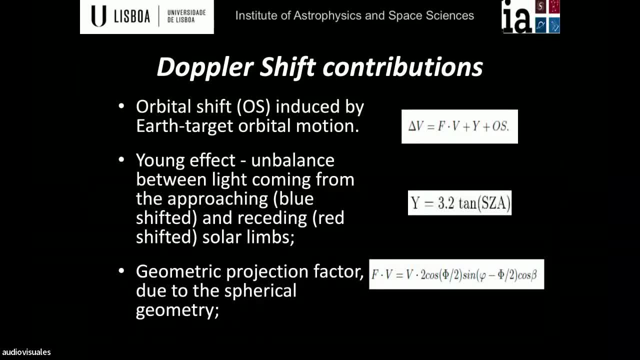 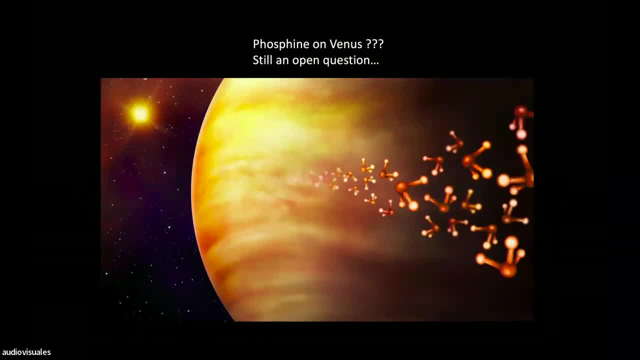 is? is that the reduction? so I think that if there is any question, of course I can go in detail, share with you what you ask, but if not, let's speak now about where I can, because I'm very interested in collaborating with you because you know much better about what I don't know, that is, the biological. 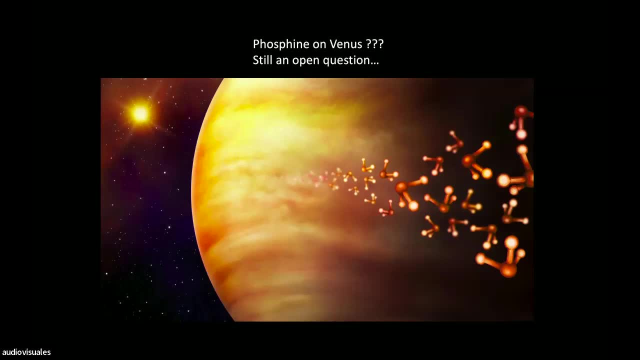 and and more chemical related with life things. so I I watched well my my years to hear from you and the kind of research you do, you do in this beautiful research center, and to see if we can envisage some line of complementarity where we can be useful for you, for instance. so, speaking about phosphine, why? 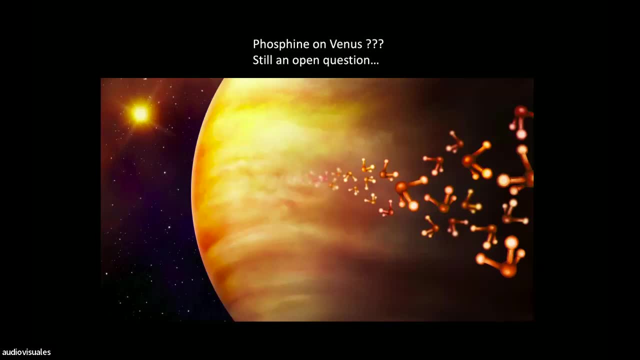 phosphine is so important. there are tons of phosphine on Jupiter and Saturn that we know even gives that reddish color. on Jupiter we are not just phosphine but phosphorus compounds, the chromophores. however, phosphine in rocky planets that we know. there is no other way of producing phosphine than our bellies. so all of 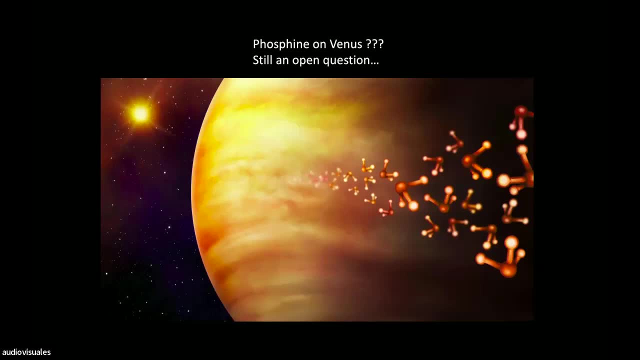 us we have- we are very rich on this because all of us we have a lot of phosphine on us, so phosphine could be used as a biomarker. of course I'm in direct collaboration with- she was from MIT, uh, brilliant scientist. now she's in Harvard and she's called Dr phosphine. she's 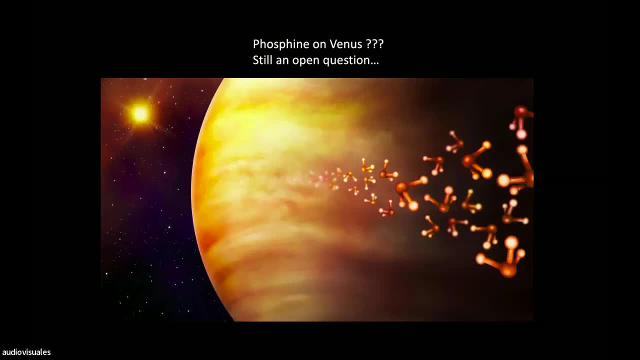 specialist in this molecule, and the thing is that could be useful for biomarking, if we learn how to do that on the solar system, even for, uh, the exoplanets. one day, with the ELT and ambition, who knows, we can find phosphine in a rocky planet, eggs or planet. well, first we must disentangle from I I often 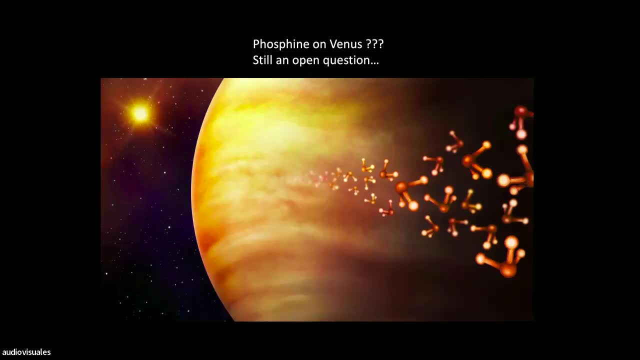 hear in the news, Earth's like eggs or planets, and I'm always with a witty card. I know I'm always not very comfortable with that. I will. I prefer to say the Venus look like, because Earth is very special. so the size we can say size of the Earth, Earth's type, uh, for me is a bit too much Venus. 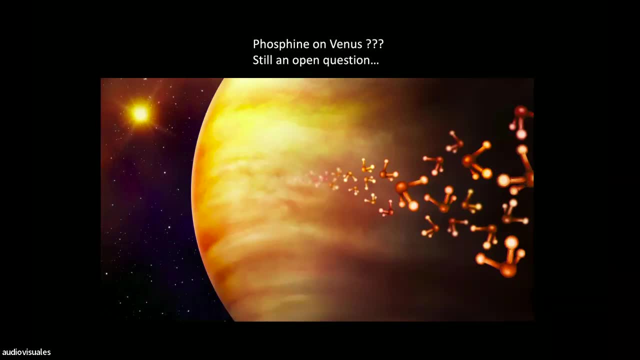 is more normal. I would say Earth is very special. so again, phosphine is very important because of this, in the rocky planets we don't know other way of, uh, phosphine, besides that very strange and weird thing called life. So and was proved that no. 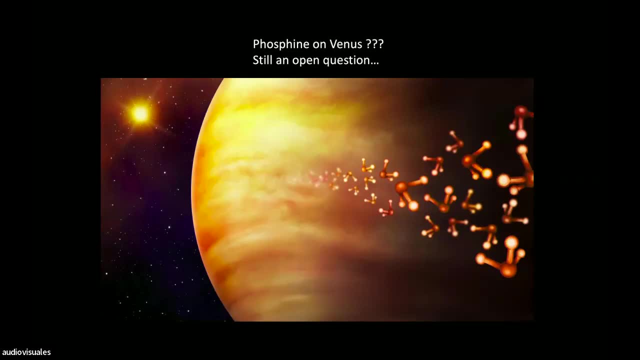 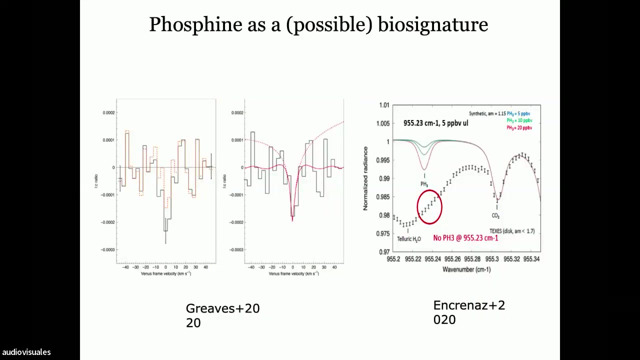 volcanism, no other sorts of no lightnings. no, It's not possible to form phosphine. We can produce in an industrial way, of course, but life is prone to produce this. So this was the first detection from Greaves from ALMA, and there is a lot of controversy about that. 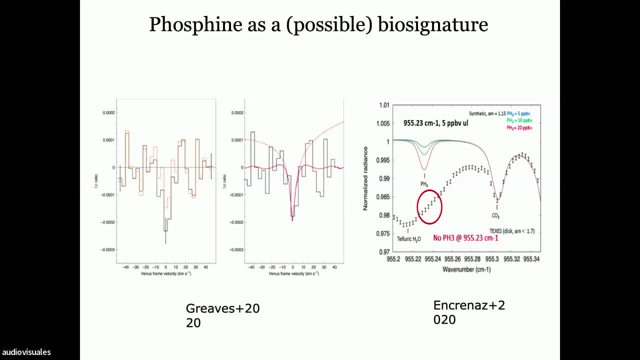 as you know, and there is a canal that we work in a close collaboration, from using data in other parts of the spectrum, not on this. as you can see the other spectral signature and there is no phosphine. I don't believe. 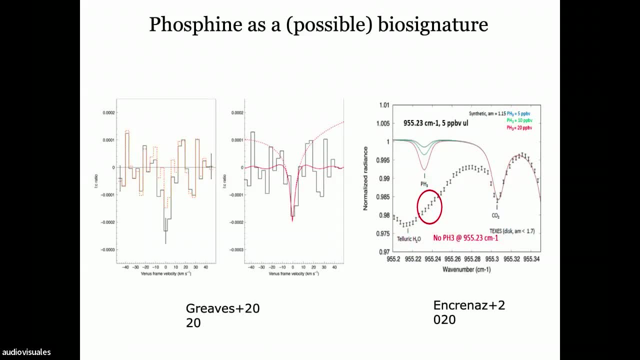 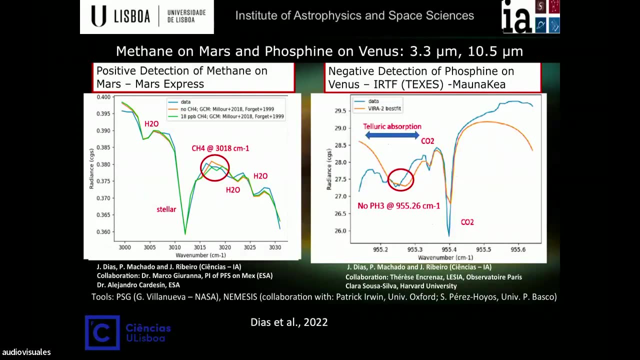 But we gained three missions to Venus. So here, what I want to show you is our trial to support the detection of phosphine on Venus. But as you can see in this our previous, and we perform dedicated observations in different regions of the spectrum and there was always a no go. That's a pity, but 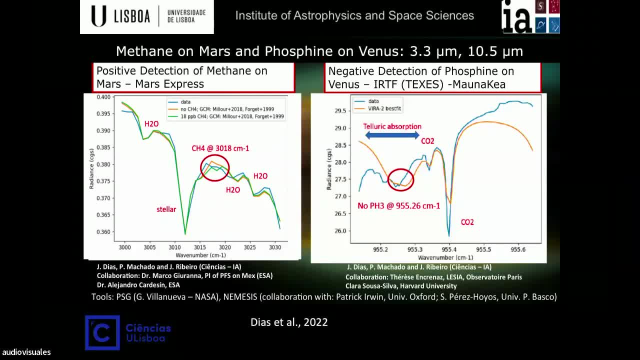 we'll have other other corps to other bodies on the solar system to study, like Enceladus, that is a brilliant case. or Europa, Ganymede, But no, go, as you saw. On the other hand, on Mars there is the detection of methane from Mars express. There were orders from the rovers. 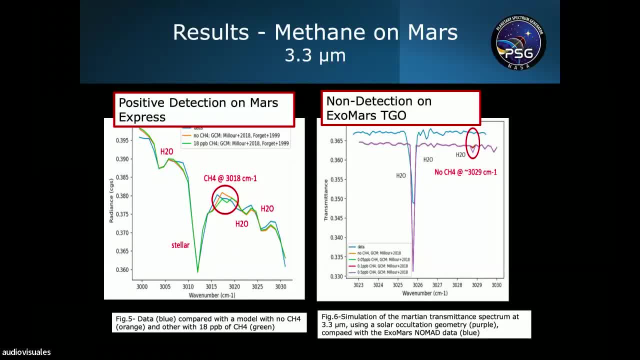 as you know. but there are also a lot of things to study about that because, for instance, there was a no go related to exomars-CGO, related with the study of this year of methane on Mars. So So we don't know. It's highly variable, It's special and temporal variable, the emission of methane. 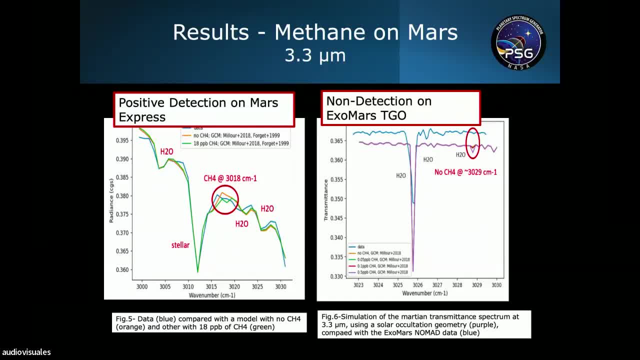 In my opinion, that fits. If it's underneath microbial life, it's possible. If it's serpentinization, as you know better than me, it's one way that we can collaborate with you That we are trying to develop a method to disentangle if the detected methane will come from a biological source or from a geological process. 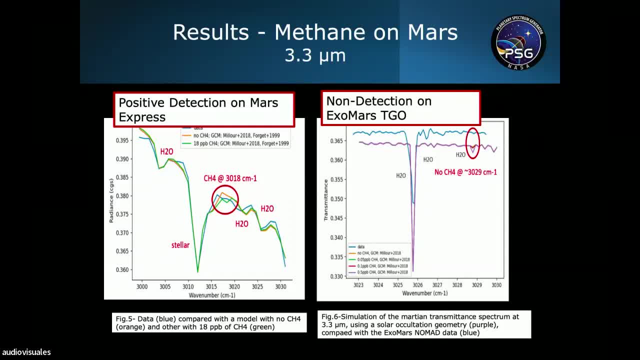 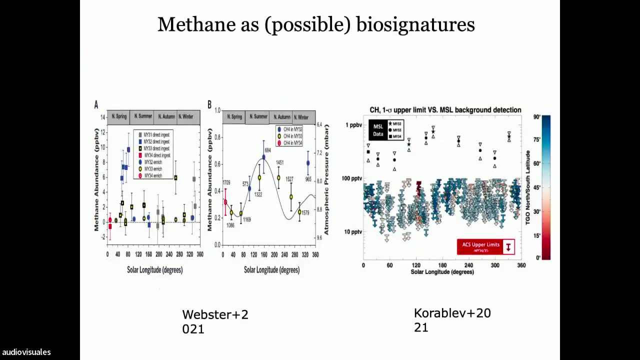 From the olivine. you know much better than me, But we are trying to develop and function this method, so we'll be open to discussion about that in the near future. So methane as possible. I think that in this house there is no point to discuss this with you, because you know much better than me about that. 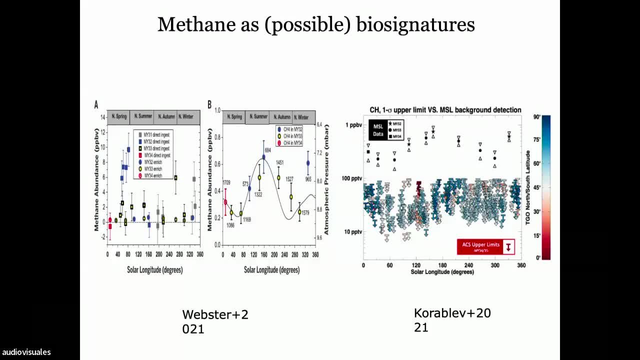 Of course, that methane, because it doesn't remain for a long time in the atmosphere, because it is fertilized by UV, so we need a source of replenishment of methane. So we need a source of replenishment of methane. So we need a source of replenishment of methane. 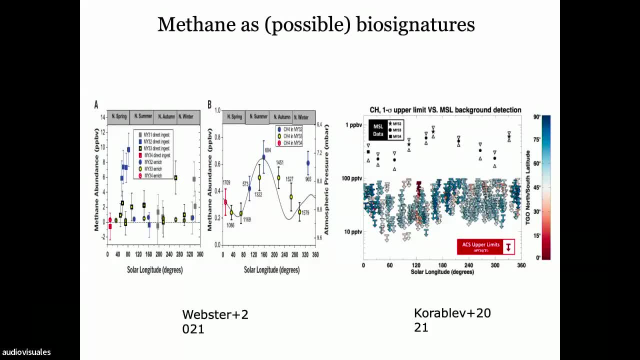 And on Earth it is the case that we know better. life is the best option to explain that. Even in New Zealand now we have a tax from the government related to its release of methane from cattle. I will not go into details because we are going to have lunch after so let's move on. 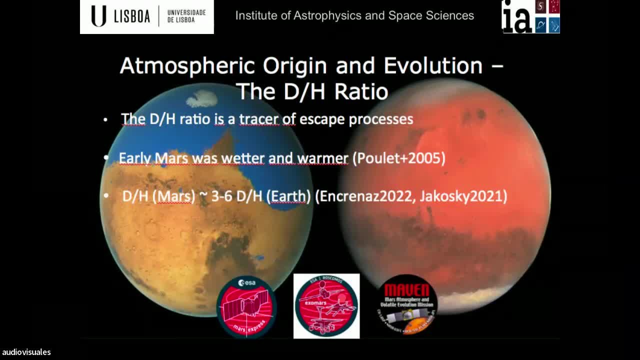 And from here, another thing, that What I'm quite interested in is to perform a compact planetology. You already saw this in between the lines on what I said till now. I love to study and compare the temporal evolutions of different planets and I have this synergy with the exoplanets we are. 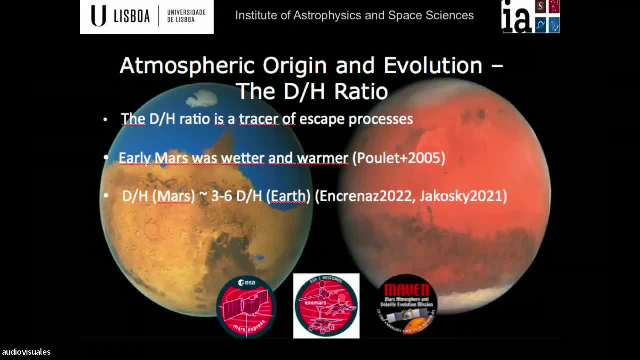